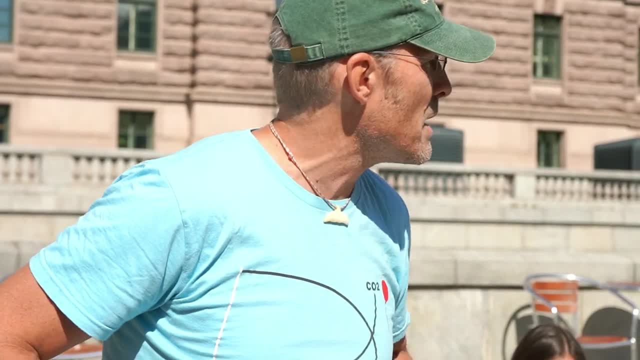 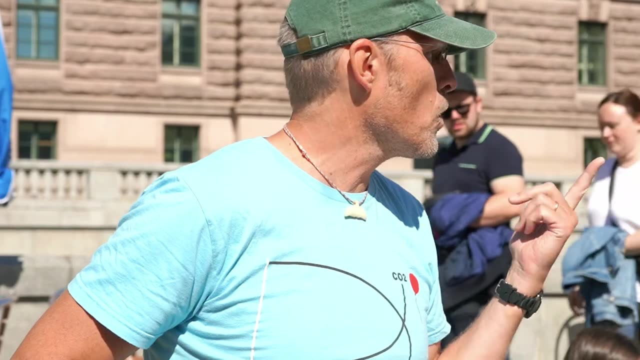 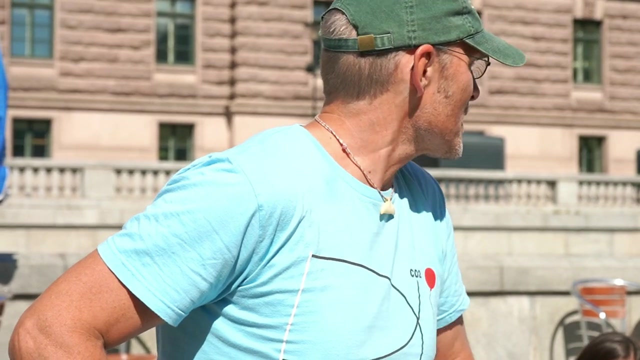 We'll talk about 800,000 years back in time. until now It's in four chapters. Who am I? You don't know me, I think. And how does a glacier work? What does it eat? What does it let out? 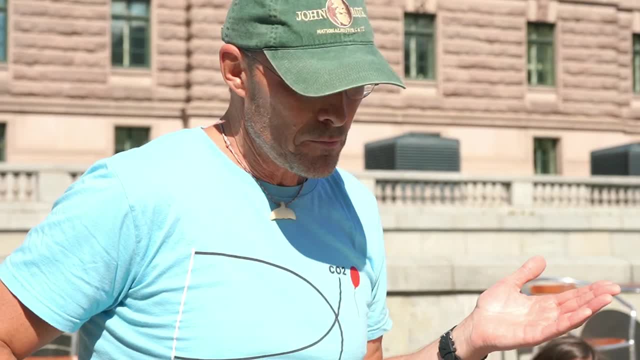 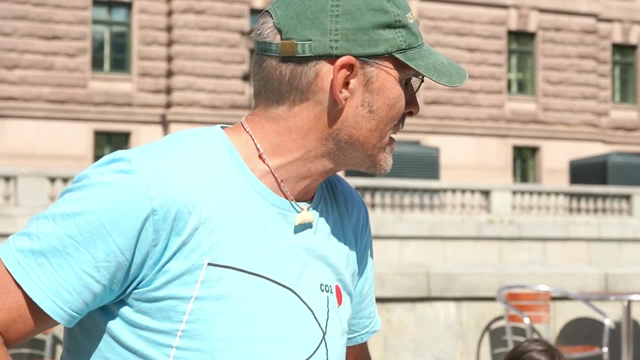 And there are different types of glaciers as well. And why do we have to care about the glaciers? They're just cold and dangerous, A lot of crevasses you can fall in and die. Why should we care about them? And then, in the end, what have we learned today? 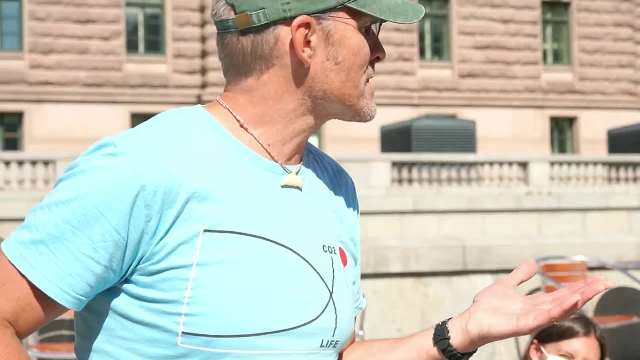 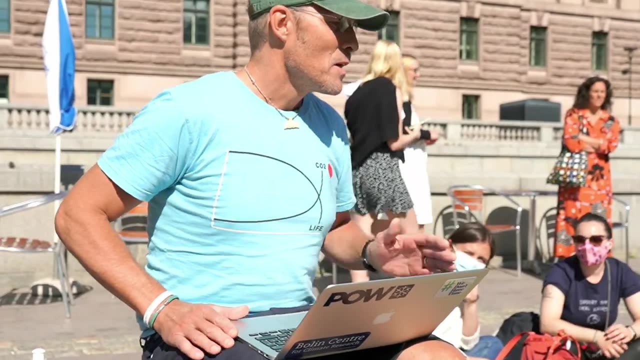 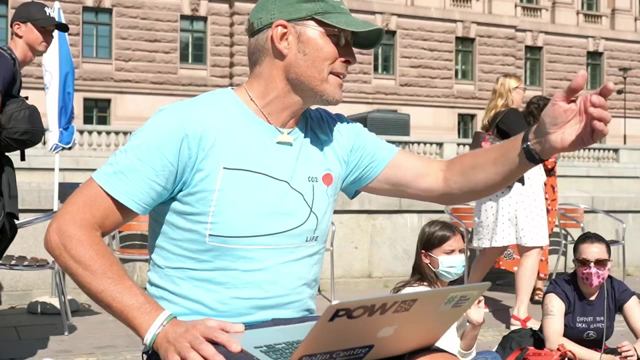 Sound okay And my voice is yeah, great thanks, A lot of fans already. So who am I Actually? when I was young, as you, I just loved skiing, have fun, climb in the mountains, And that's where I met Toya 150 years ago or so. 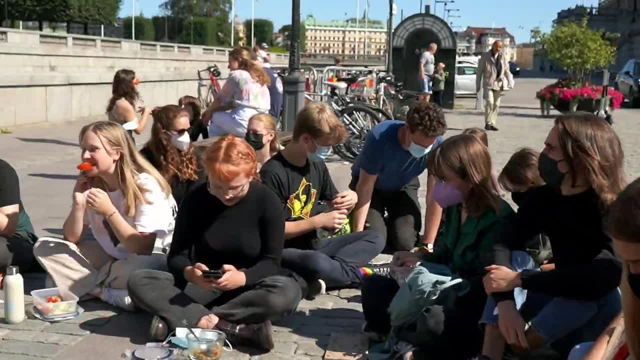 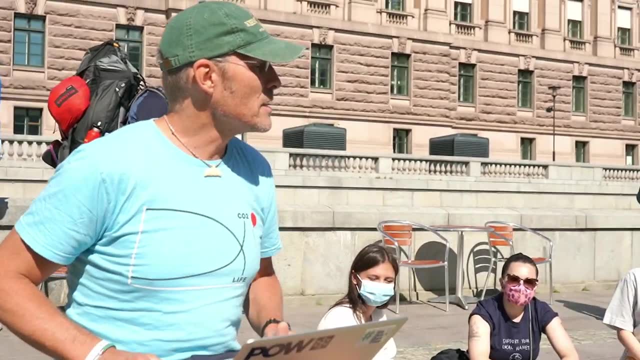 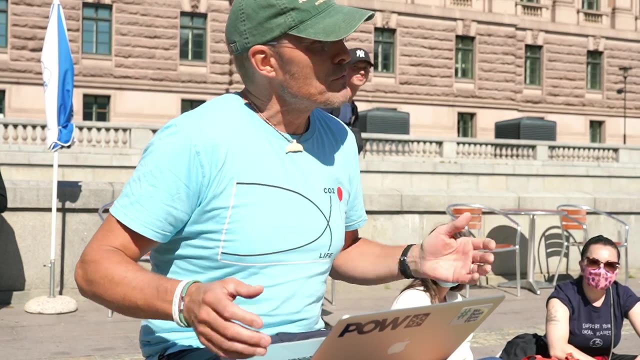 At least Talk to yourself. Yeah, So we went down into the Alps. We took the train. of course, Nobody could board an airplane by then, And it's a lot of seasons. We were skiing and we had actually some serious accidents with avalanches, but we survived. 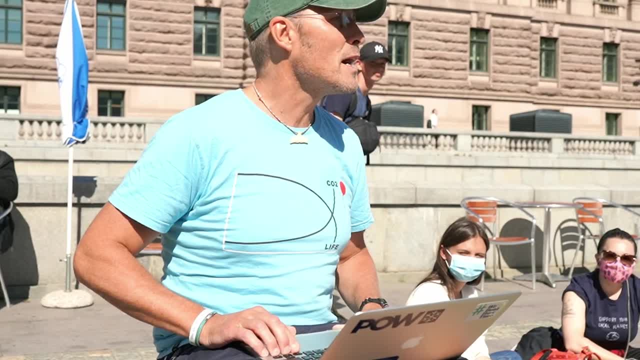 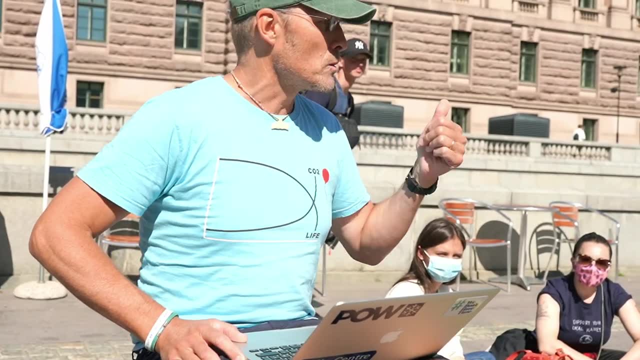 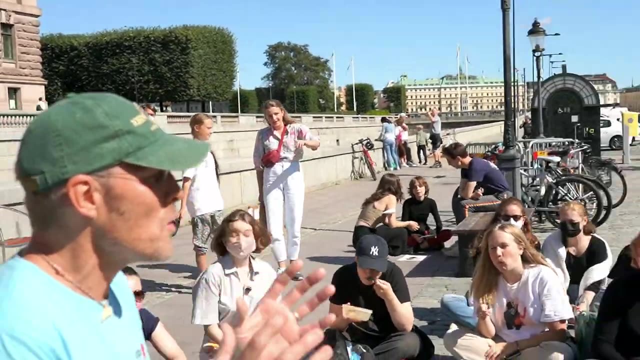 So we're still alive. But finally, I found this topic- geography- in the university And I started to study that. you know deserts, tropical rainforests and glaciers, And I found that- these glaciers. I was so fascinated by them. 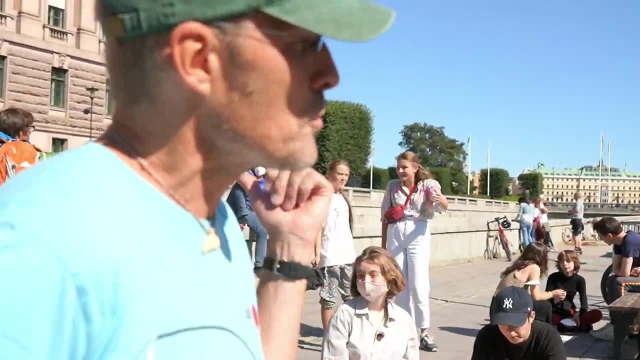 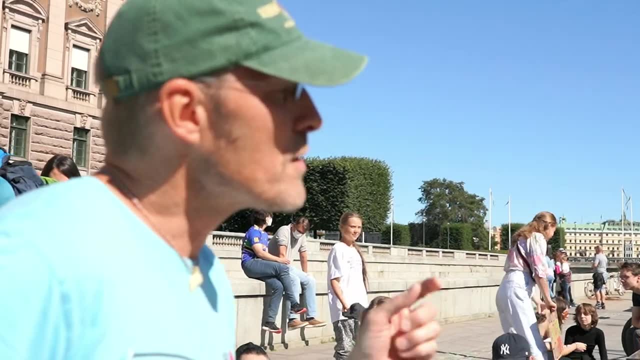 So I had to study them more. So I went up to Stockholm University And they have a field station up in northern Lapland. It's called Tarfalle Research Station. It's very close to Kemnekäise, which is actually still the highest mountain in Sweden. 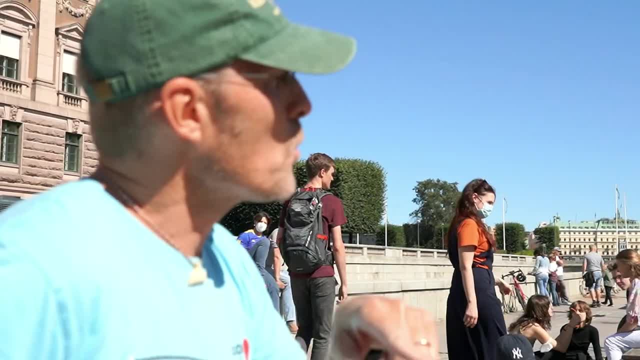 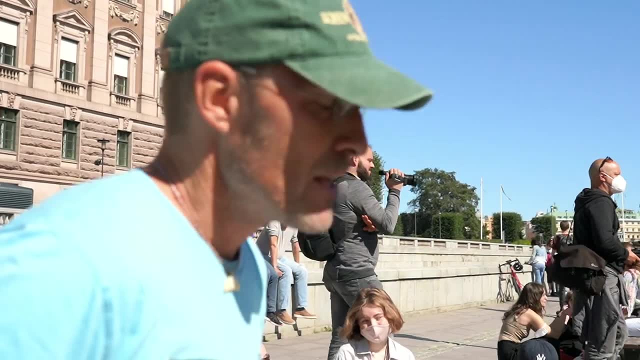 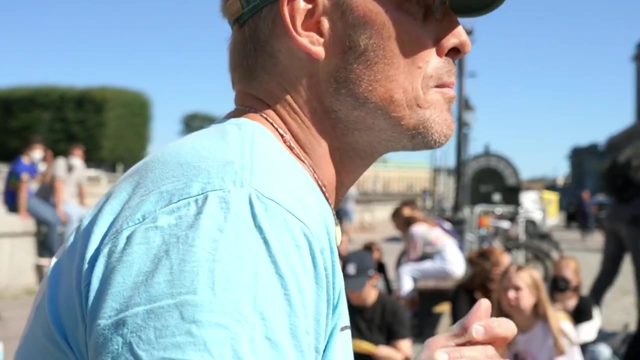 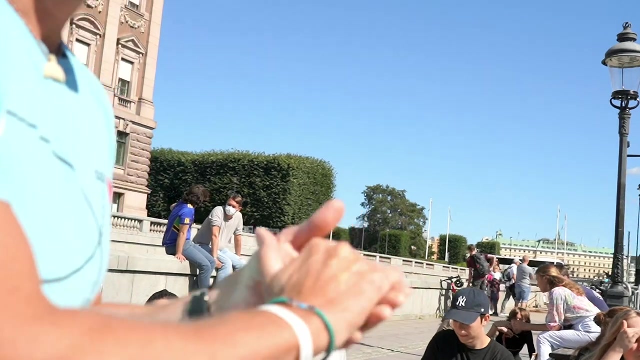 Not the south summit, because it's melting, but the northern summit, And so that's what I've been working with most of the years. The latest years I've been working with Earth System Science and Communication And also business development to help companies and organizations to adjust their way of working in harmony with the planet. 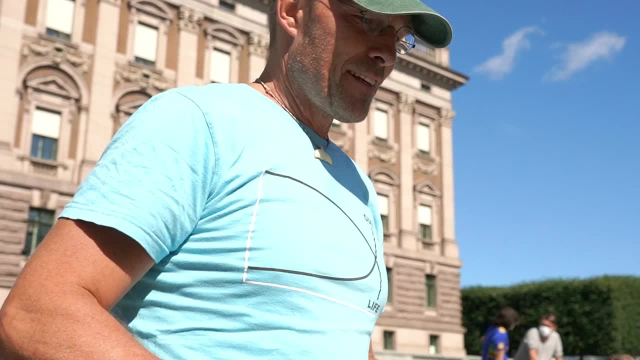 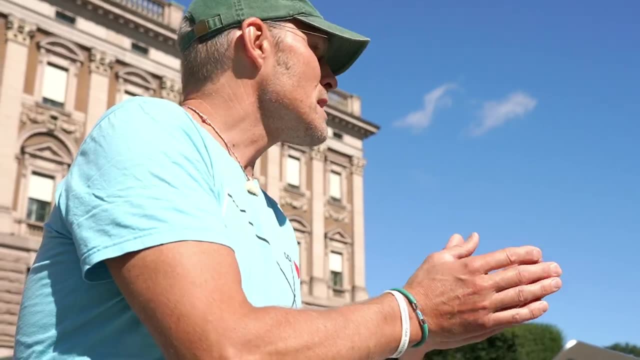 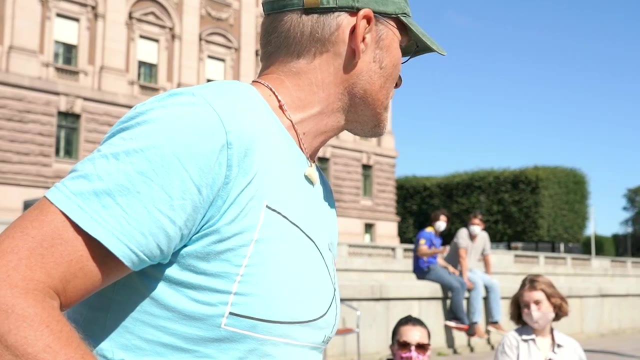 So we'll go further on. So my office for many years was in Kemnekäise Mountain. It's a little valley. It's five glaciers all around there And you might be surprised that in Sweden we have 250 glaciers. We had 300 in the 90s, just 30 years ago. 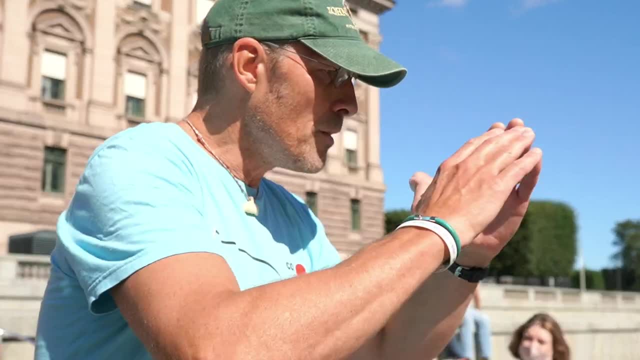 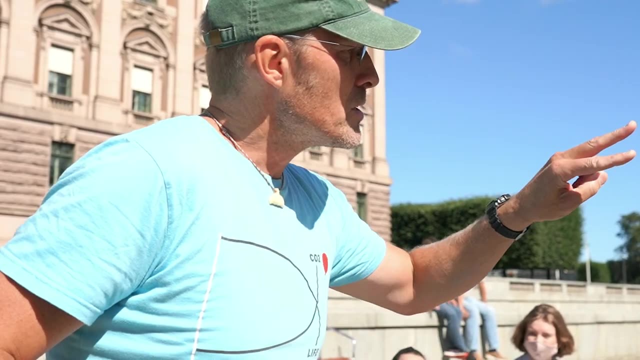 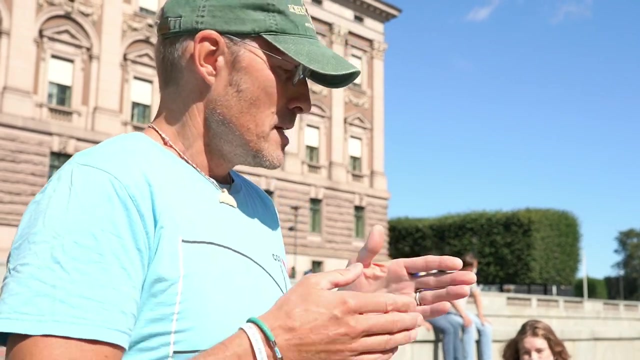 But now we have 250 left And they are decreasing very much. And the south summit has melted two meters since last year, So now it's two meters lower than the northern summit. So if you want to go up the Kemnekäise Mountain, you have to climb on a ridge with rope, ice axe and crampons on your feet. 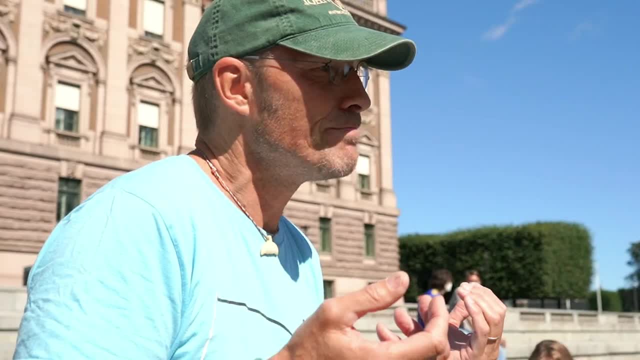 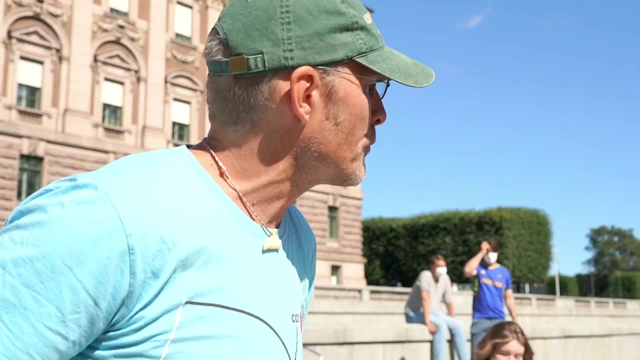 And probably have a guide. So it's a bit more difficult If you want to go to the highest summit. So to work on a glacier, you have to be careful, You have to have a rope, crampons and ice axe And to be at least three persons in the rope. 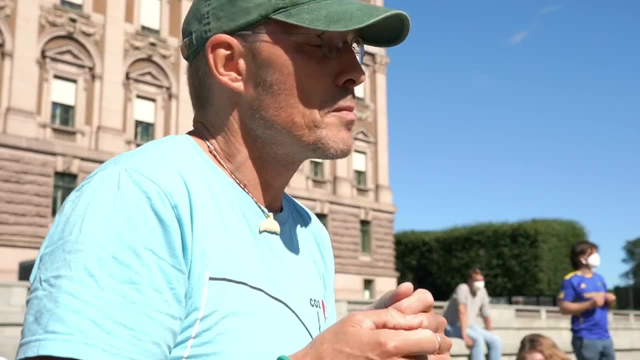 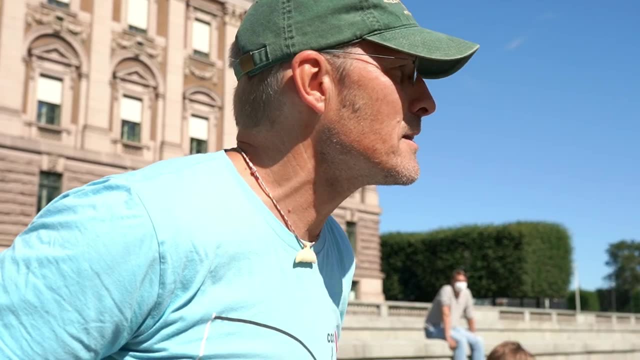 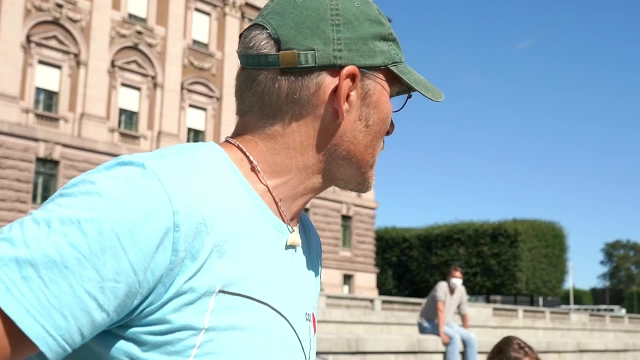 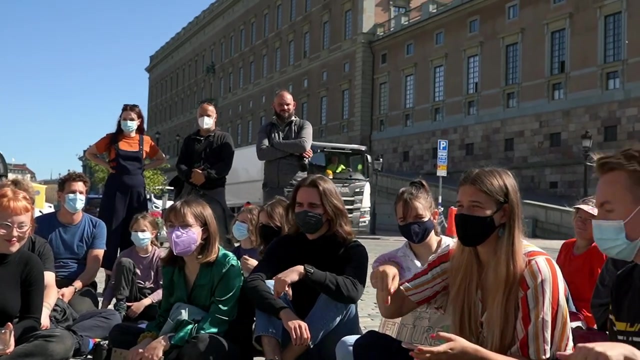 Because if someone falls in or to traverse, you have to be able to drag someone up. In the early 90s, I was invited by a professor to work in Antarctica. Where is it Point at Antarctica? everyone, It's down there. 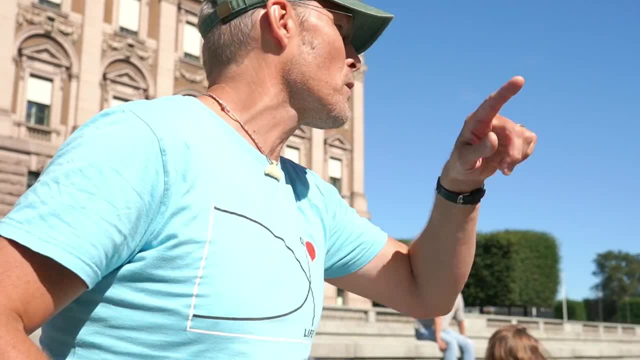 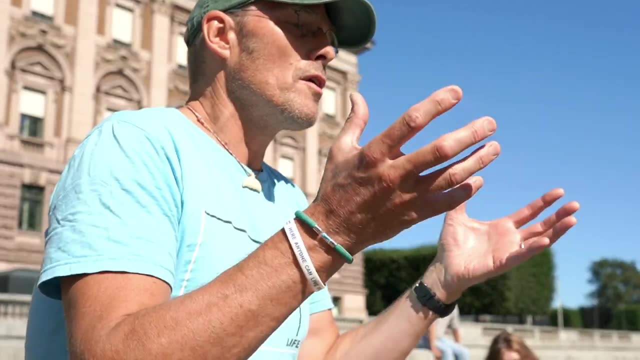 It's about 7,000 kilometers to the earth, But you can go on the surface. So I was there in the early 90s drilling ice cores, And we were preparing for a big drill project That resulted in the deepest ice core ever made. 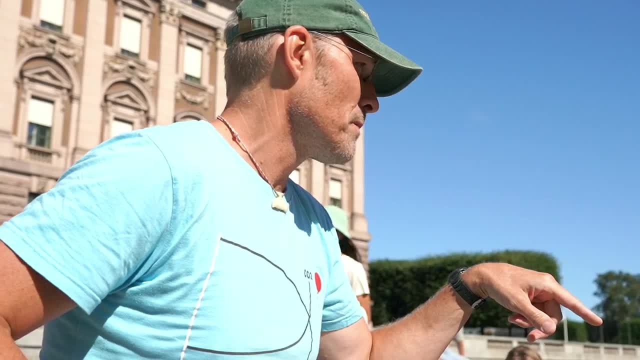 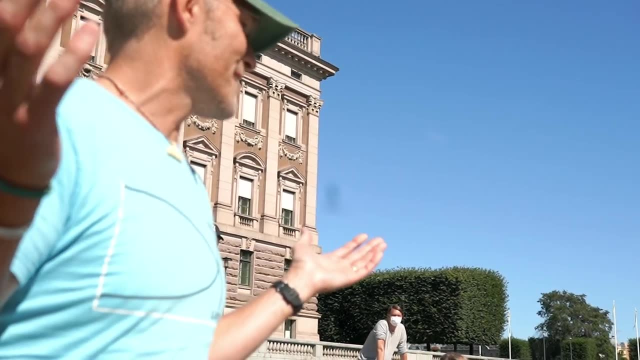 It came back eight ice ages back in time, So it's 800 years, 800 years back in time. So why do we do that? Why do we drill in an ice sheet? It's 4,000 meters deep. Well, in these ice cores you have small bubbles. 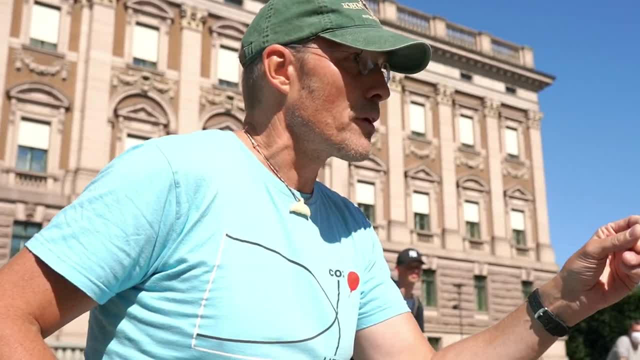 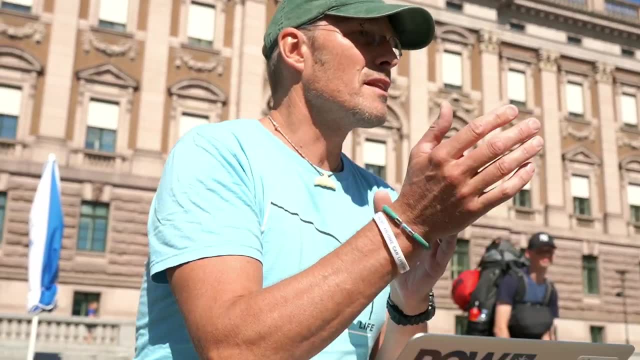 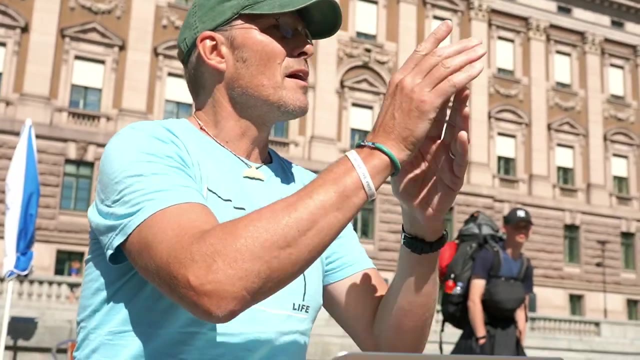 And these bubbles. they consist of air atmosphere from that specific time And by analyzing that atmosphere you can see what was the composition in that time And what was the temperature. So you can use the oxygen isotopes By creating a temperature curve back in time. 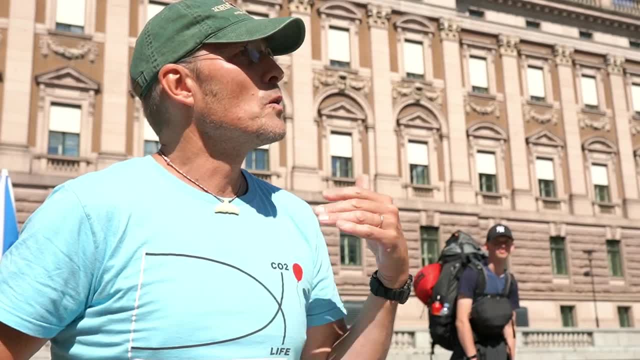 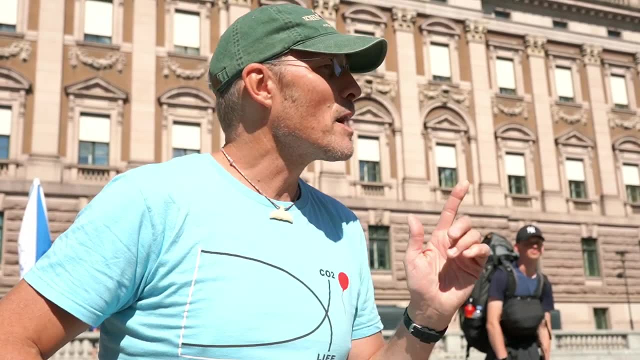 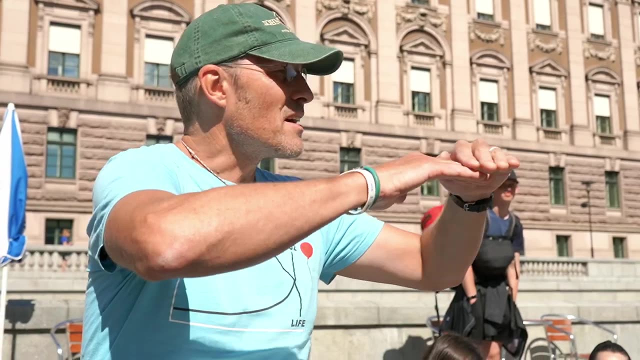 It's called a climate proxy And normally we didn't have thermometers 500,000 years ago. But we have the glaciers, Perfect archive. And in Antarctica the ice doesn't melt in the middle, It just layers, layers. each year new layers. 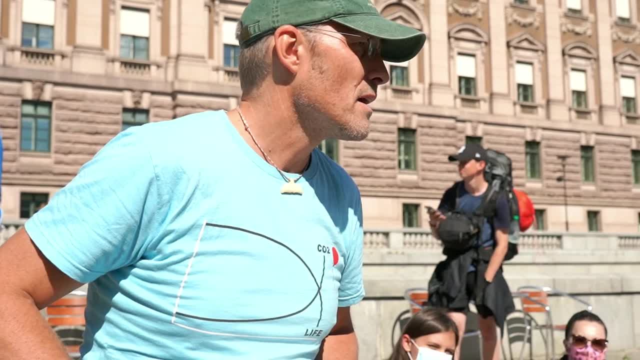 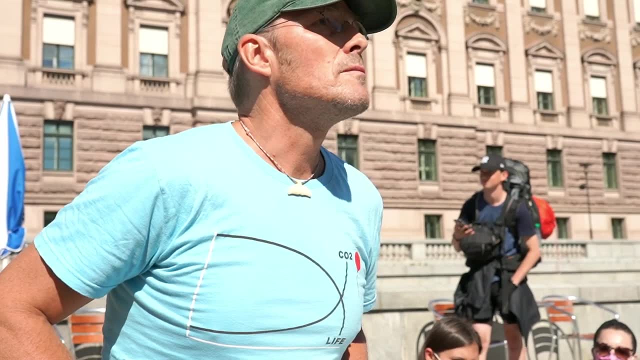 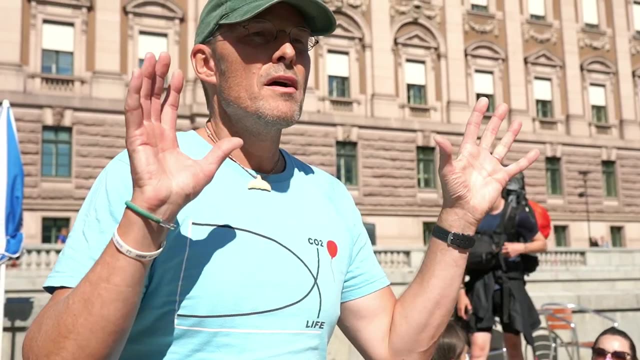 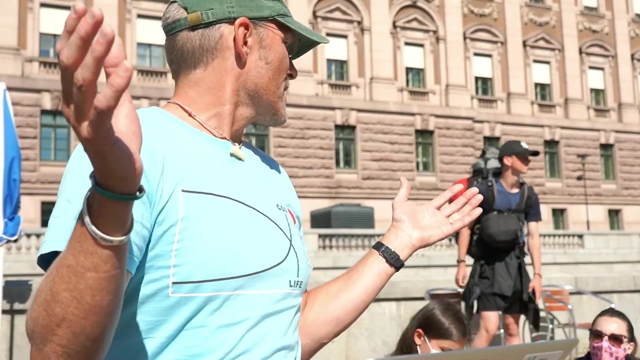 So that's how you can analyze the glaciers, But they are actually drilling a new core. now That will become one and a half million years back in time. So the last two million years we had around 20 ice ages, And the normal stage for this place is ice age. 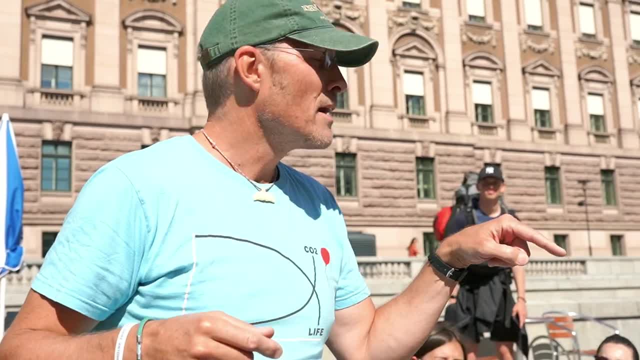 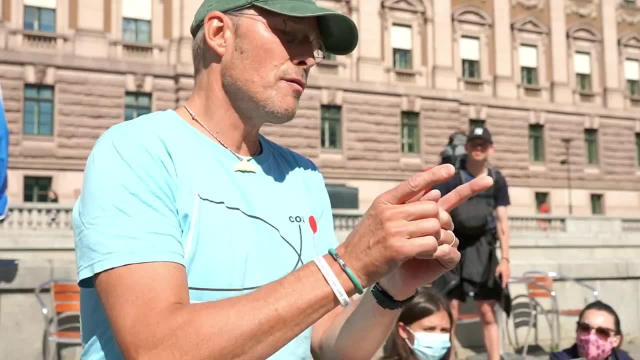 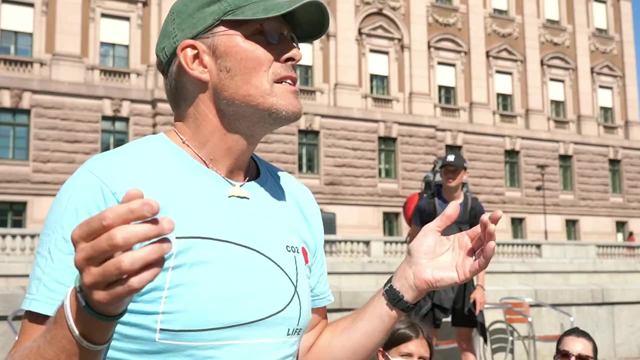 That means we have three, four kilometers of ice here, And this is 500 meters below sea surface. That's a normal situation for Stockholm. Now. we live in an interglacial between two big ice ages, So we have this warm, pleasant weather. 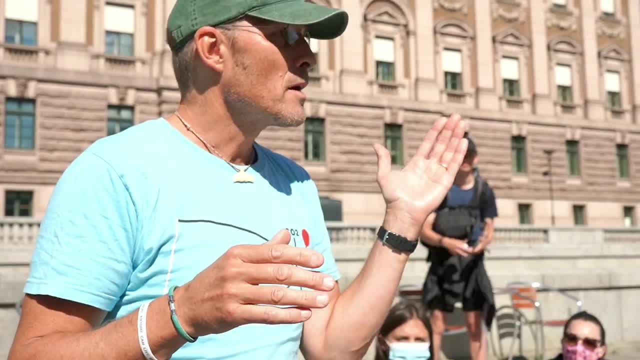 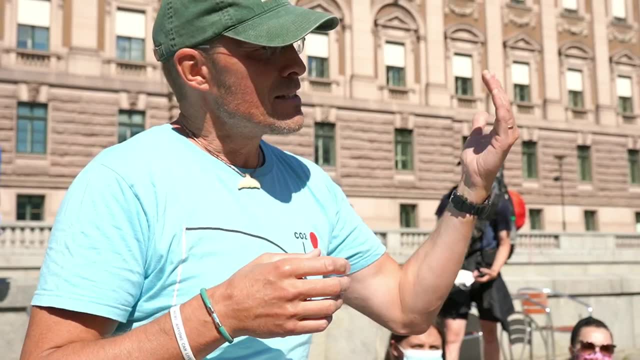 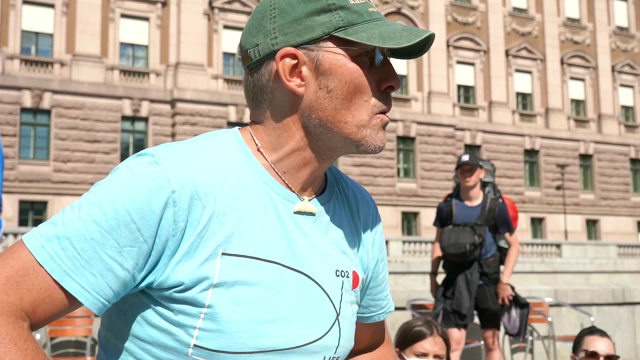 Slightly too warm, Slightly too fast warming, But it's between two ice ages And now, when the last ice age when we had, that was about 20,000 years ago- The sea level was 120 meters lower than today. 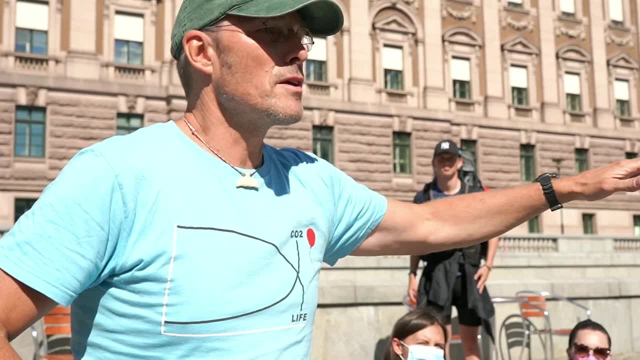 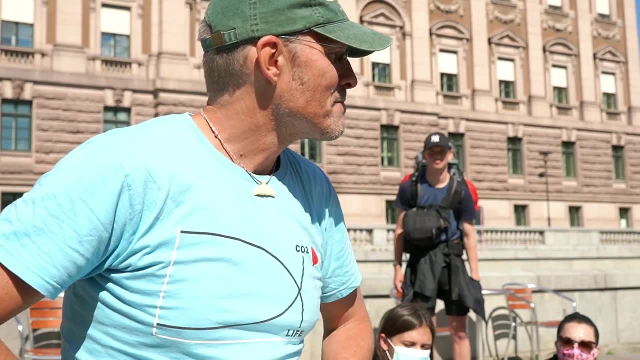 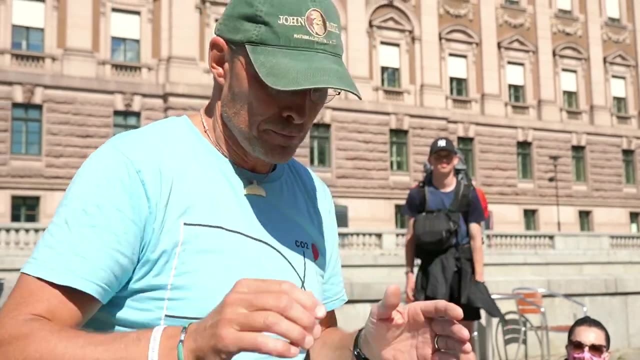 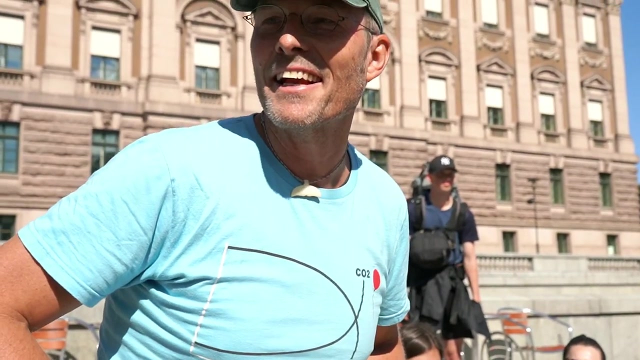 So imagine the whole northern sea. It wasn't the northern sea, It was a big landscape with rivers and fields, So it's hard to imagine. You know, nature develops really fast with ice, And so what is the glacier? I should have said that in the beginning. 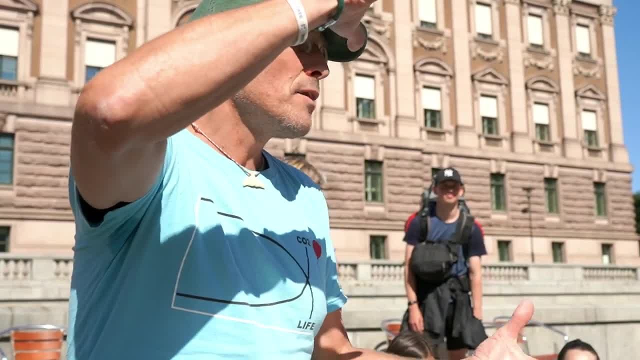 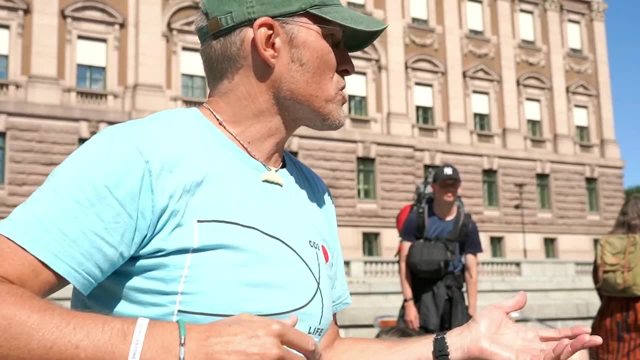 It's a huge piece of mass that is so thick that it moves by its own weight. So if you just have a snow patch that is 20 meters deep and it doesn't move, there's no ice in it, it's no glacier. 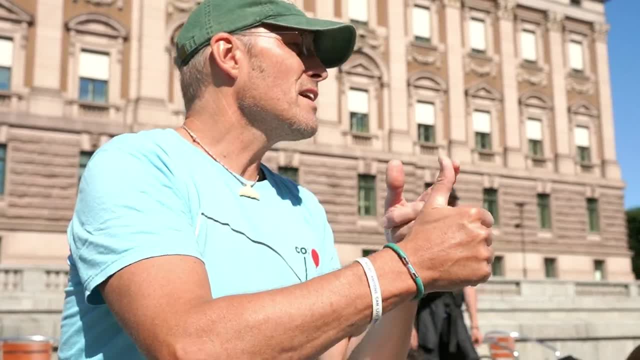 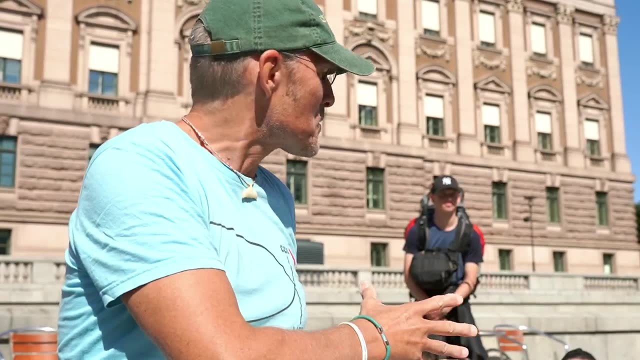 But when it starts creating ice where air and water cannot run freely, and it starts moving in a plastic movement, it's not elastic because it doesn't rebound up to the mountain, And it's not vicious like a river, But it's plastic. 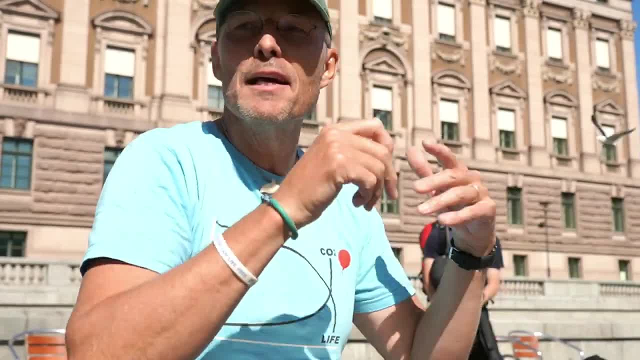 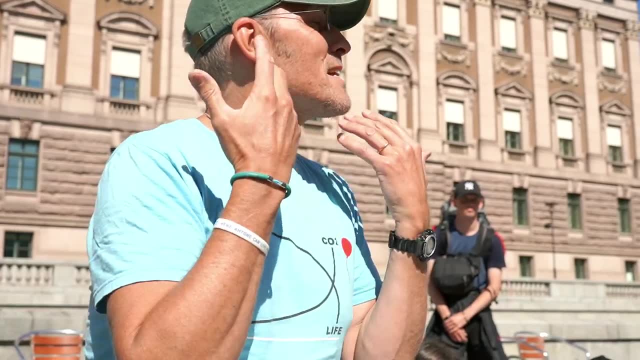 It moves like a dough. You know where you make a cinnamon bun. It's like that. But no cinnamon, no sugar, Only snow. And glaciers they love snow, And when it's too hot they melt. So that's how the mass balance works. 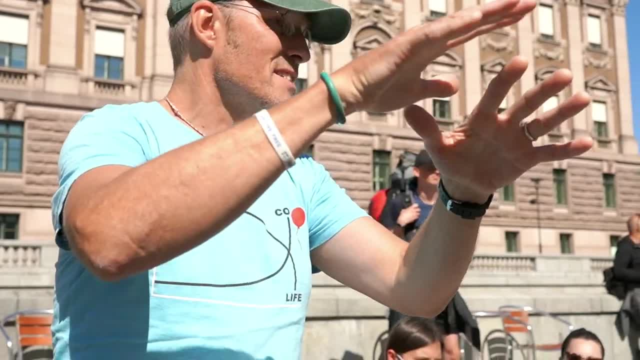 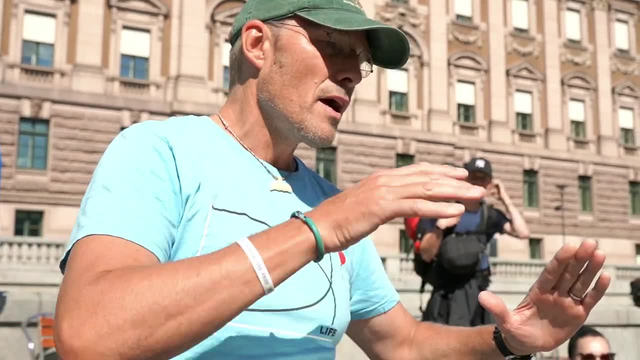 You fill up, they eat snow and they create that to ice, and the ice moves through to the front and then it melts. So the front is melting more and more and the top is getting thicker. So if it wasn't any movement in the ice, 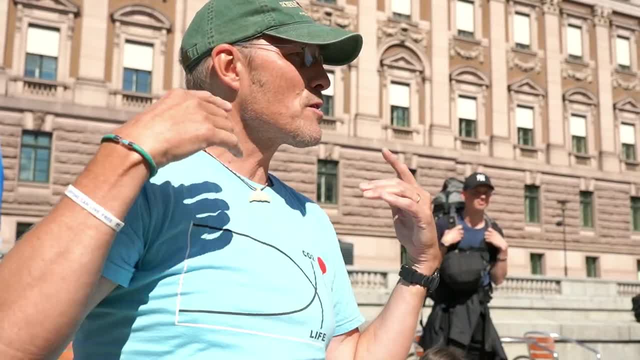 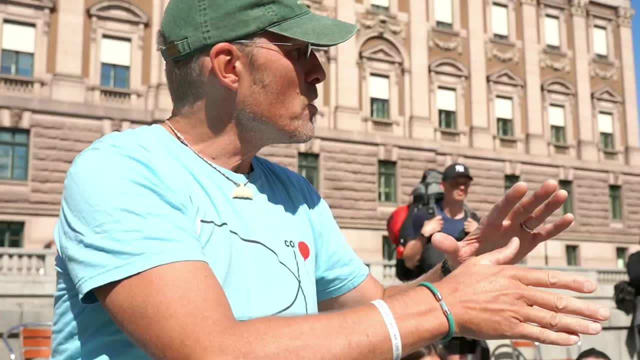 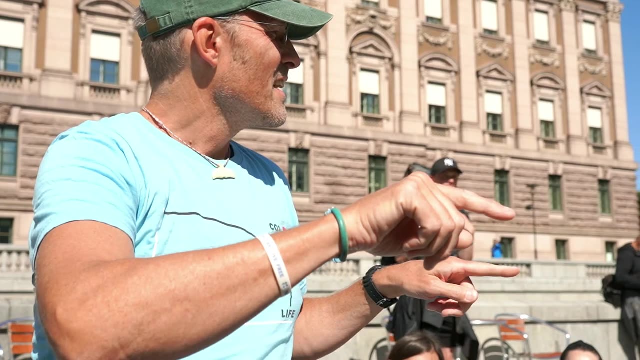 then every glacier would just tip over. But you have this thing called gravity. You all know that Gravity makes the weight create the movement through the glacier. So if you drop something in Kebnekaise up there, it takes maybe 2,000 years for that little piece of. 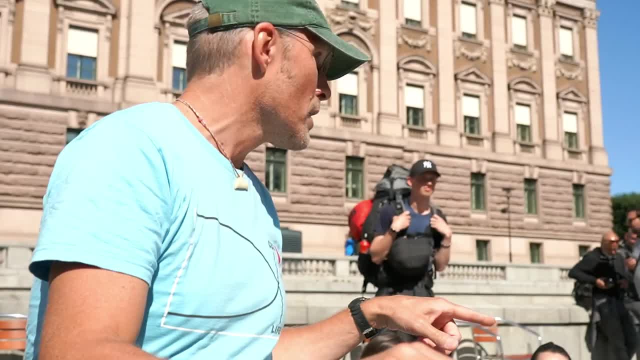 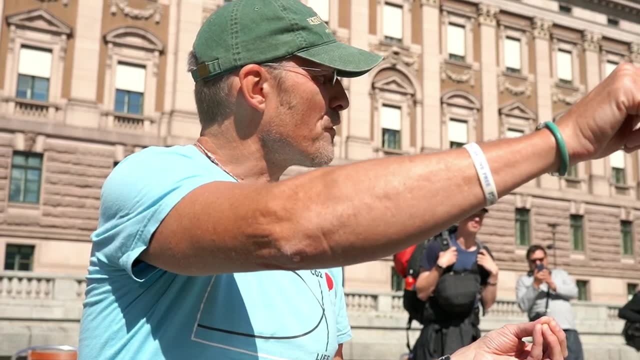 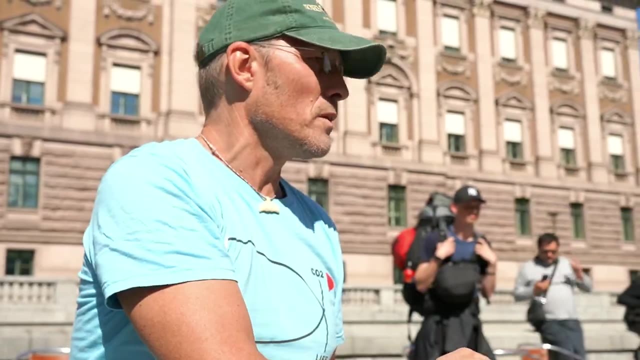 I don't know backpack or something to come up in the front. So what we are seeing in the front, these pieces of animal and stuff that was landing on the surface when Jesus was born, And in Antarctica you have several hundred thousand years of ice. 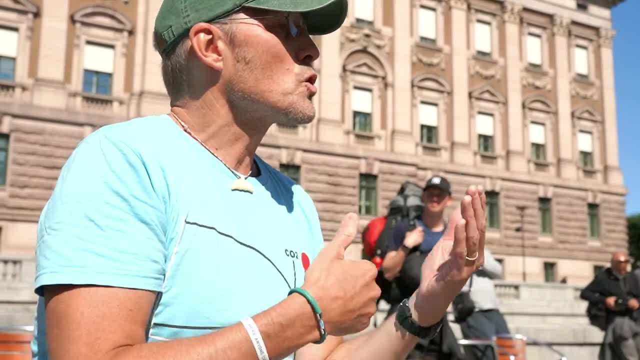 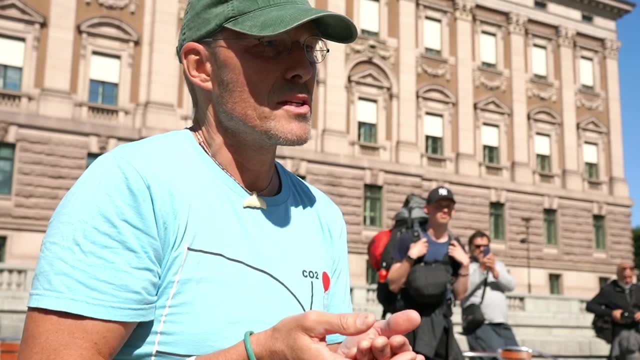 So it's pretty astonishing. It's like the glacier. it's talking to us. The whole nature is talking to us, But you have to learn the language. That's what you do as a glaciologist: You learn the language and then you can interpret what the glacier is telling you. 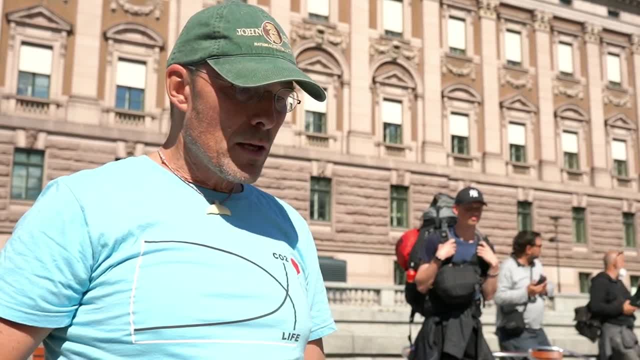 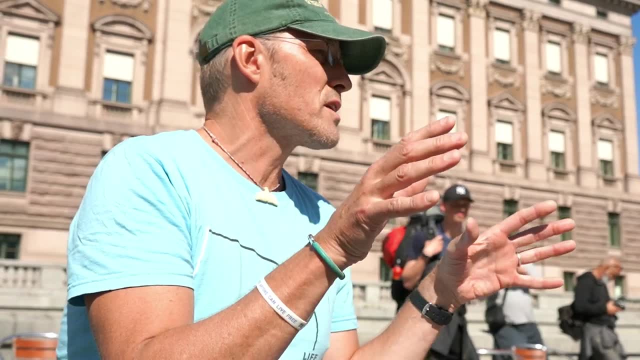 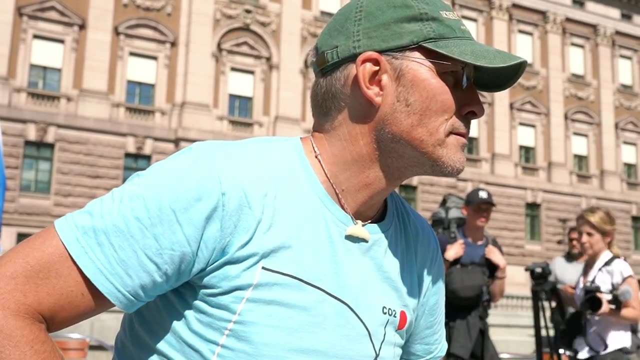 and by doing- And I give you some cold facts- as we say in my branch, So about 10% of the Earth is covered by ice, 10%. pretty much It's about if you have a big sleeping room, that's a whole bed in a sleeping room. 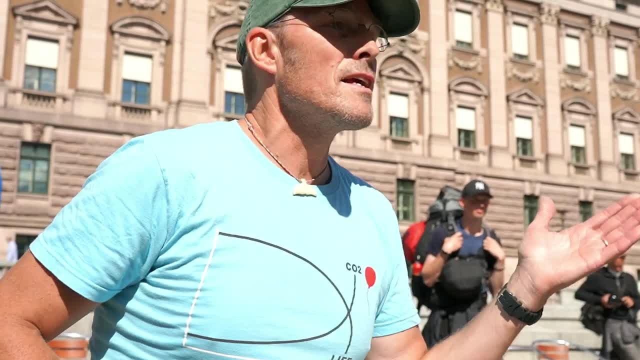 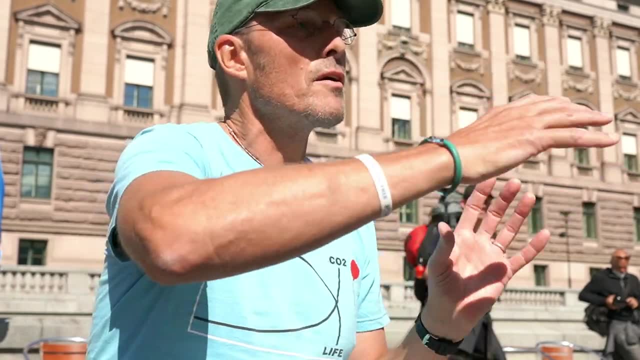 Well, 91% of the ice is in Antarctica, Because Antarctica it's a continent. It's not like Arctic. Arctic, you know, it's floating Sea ice. And then you have Greenland. Greenland is an ice sheet, But Antarctica it's the same size as the whole Europe. 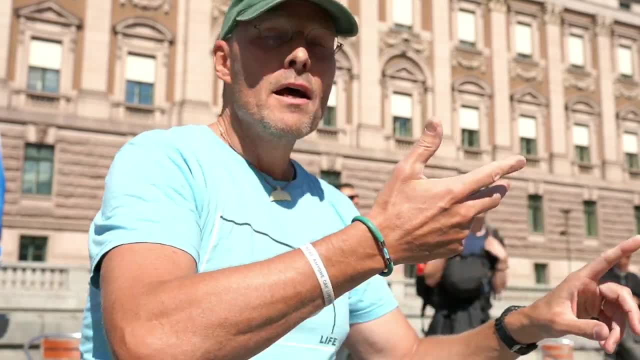 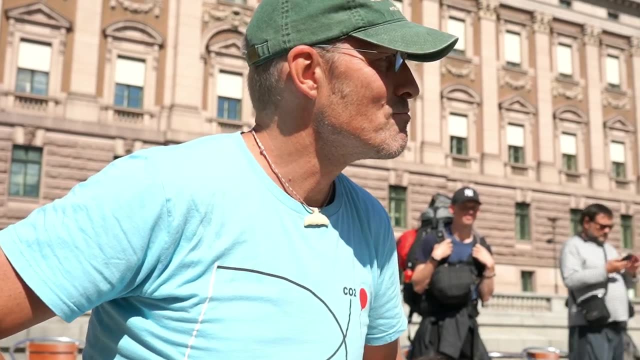 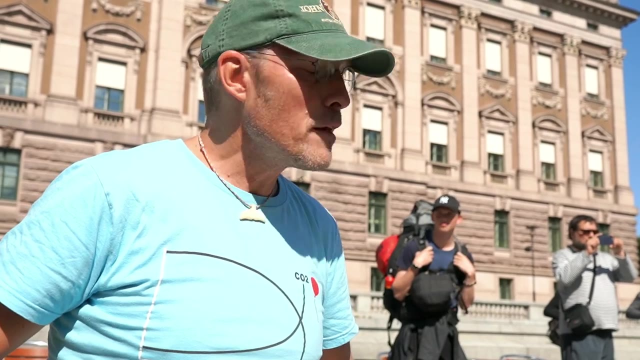 whole Northern Sea, the whole Mediterranean and the whole Russia until Ural Mountains, Just three, four kilometers thick ice. So if you're lost there, it's a long way back home And three quarters of the whole fresh water resources is in the ice. 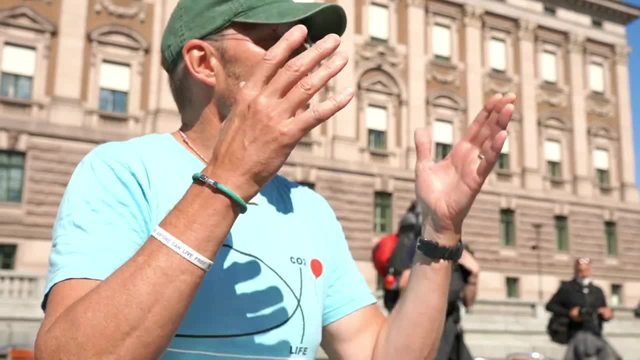 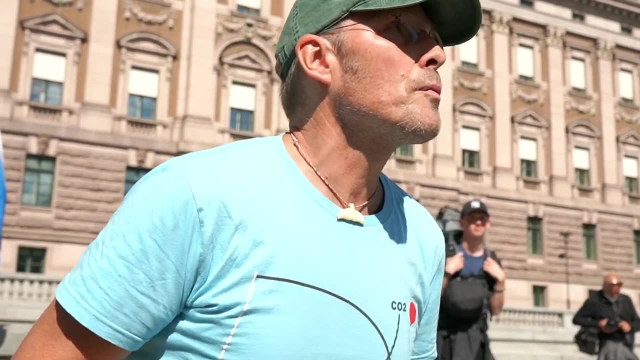 It's really important to save the ice, Because when it's no rain, you need the melt water from the ice And if, let's say, if we continue burning fossil fuels, then the glaciers will melt. They're melting really rapidly now. 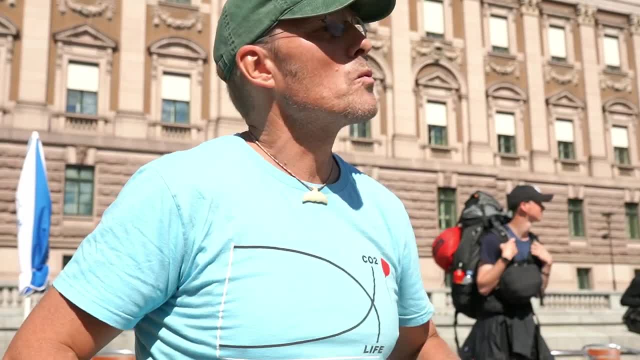 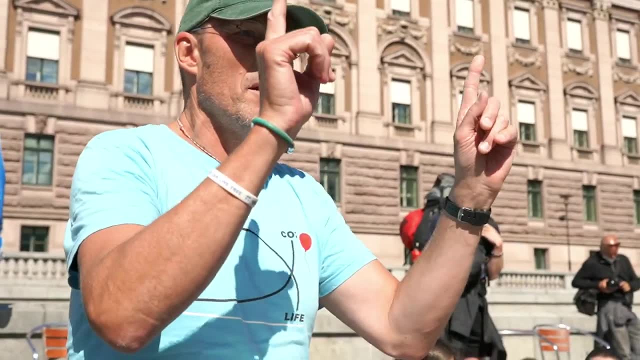 If they all should melt, then the sea level would rise about 70 meters. That would cover the whole Stockholm. The only thing in Stockholm that would point up above sea level would be Kocknäs, Tornet and the city hall where they have the Nobel Prize ceremony. All rest covered. But when it was the last ice age, just 20,000 years ago- that wasn't long in a geological perspective- Then 33% of the Earth was covered with ice- Three times as much. So it's pretty much. 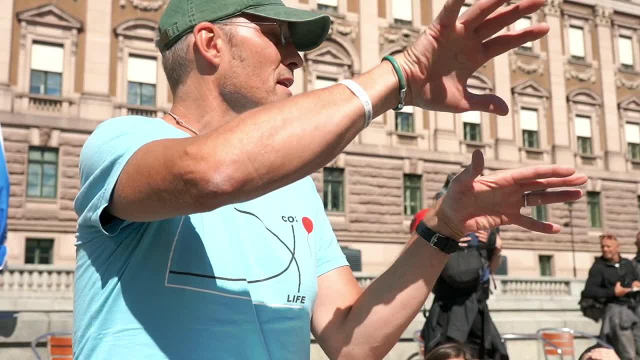 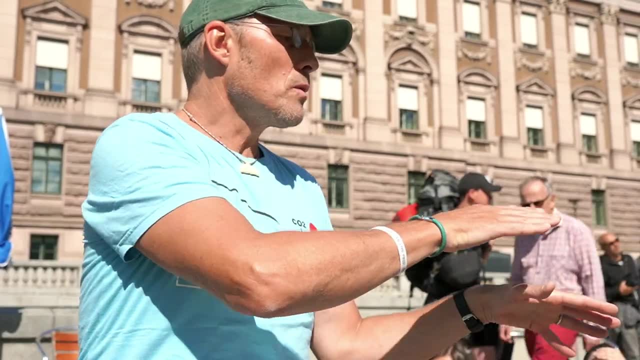 I talked about that. Now we have. you know, I talked about the glacier, how it moves. It eats snow, creates two ice, it moves and melts in the front. So you have all these movements, you have an equilibrium line in the middle of a glacier. 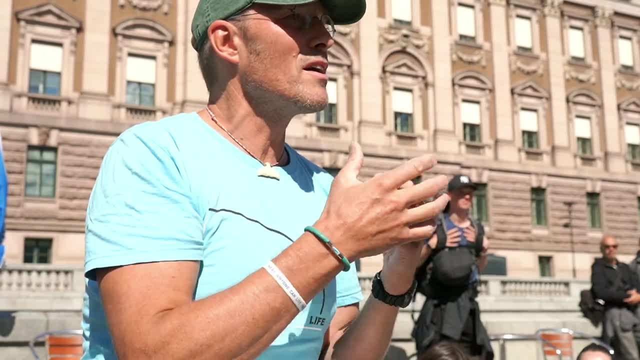 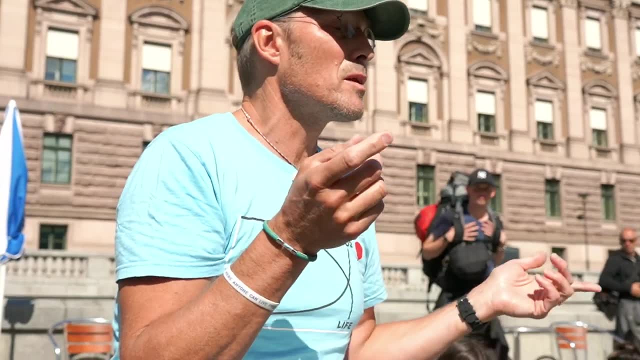 So why are glaciers so sensitive? They are like an indicator for climate. So, for instance, now we have 1.2 degrees warmer than a little bit more than 100 years ago because of our emissions. So now this equilibrium line when it's no melting. 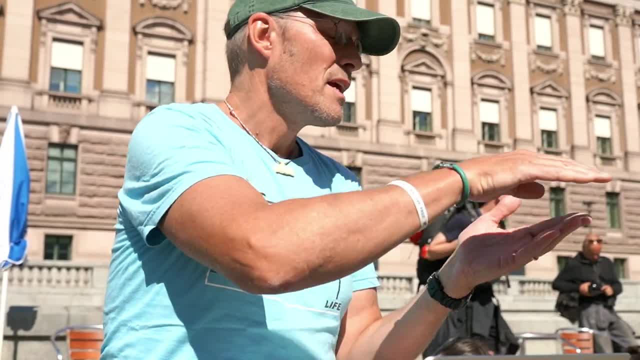 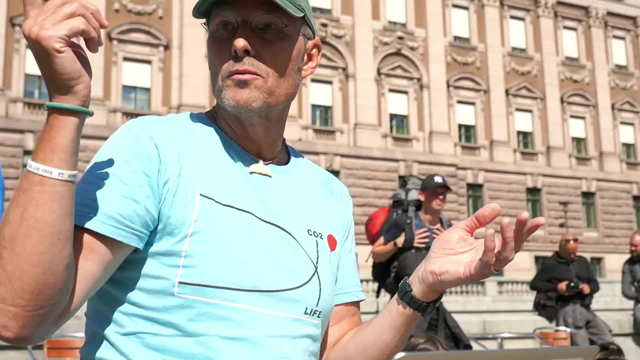 no plus, no minus. It has rise. you know, the temperature decreases, but one degree per 100 meters in the mountains. So if you go up in the mountain thousands of meters up, it's 10 degrees warmer, colder, sorry. 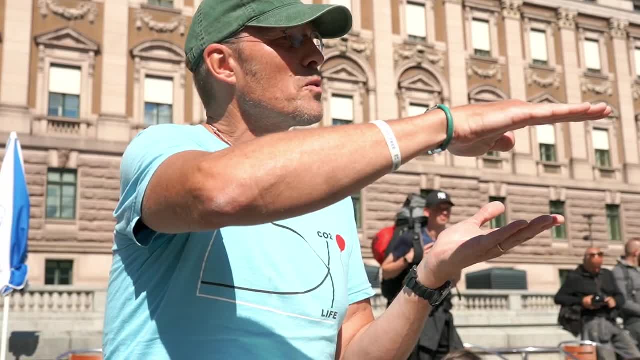 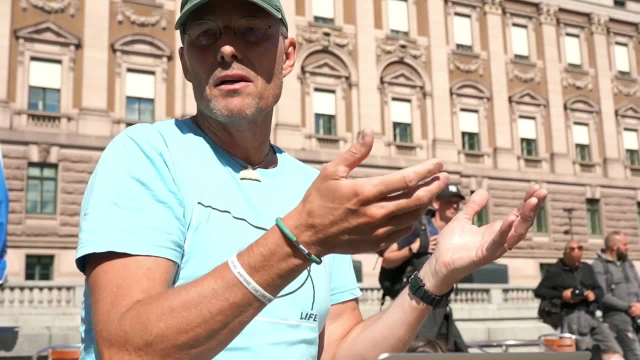 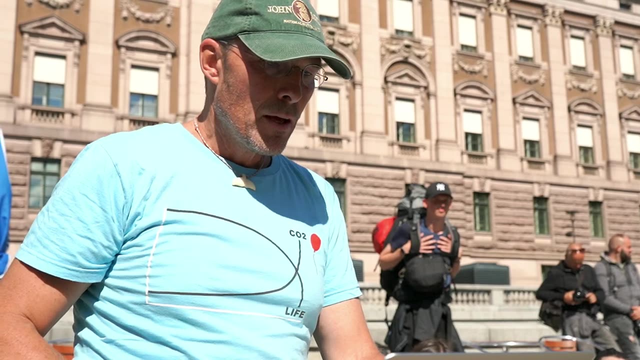 So this equilibrium line had rise 120 meters above you know, the last 100 years. So that means a big chunk of ice is melting right now. So that's the change of an equilibrium line. It's why it's melting. Then you are. 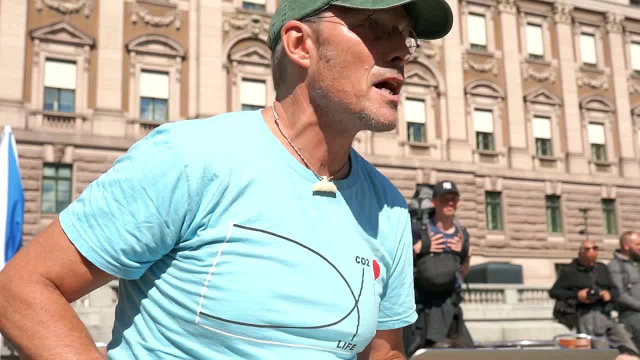 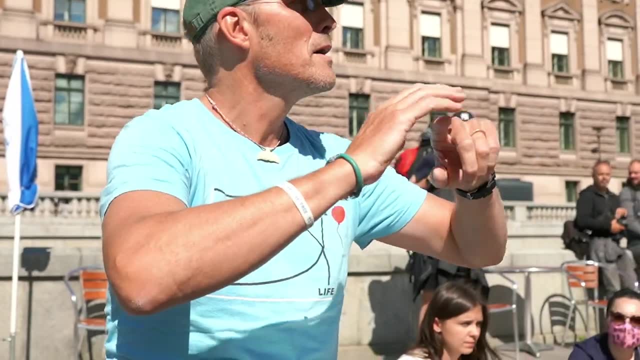 you can see the pictures later on. It's different type of glaciers. You have a top glacier. that's the summit of Kebnekaise. It's like a pyramid. You can go up there and you see 11% of the whole Sweden from the summit. 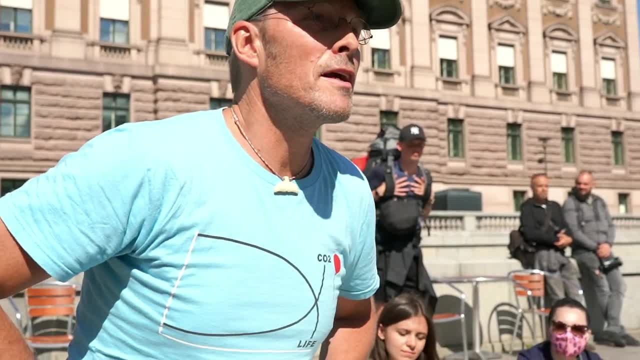 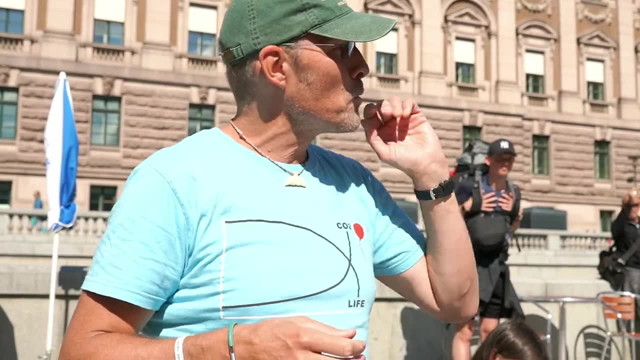 It's really beautiful. I was there last week and we were lucky. You know the groups before us. they were rushing, They had bad weather. We took it easy: took some fika, drank some water and when we came up, 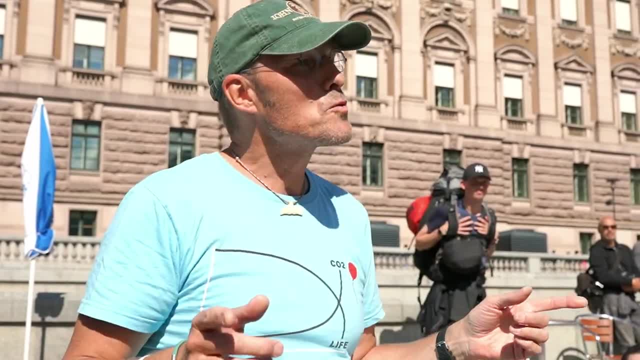 it was sunlight, So don't always rush, Wait for nature and it shows the best side. And then here you have a niche glacier. that's a cirque glacier in a little bowl. That's very common. Then you have a valley glacier. 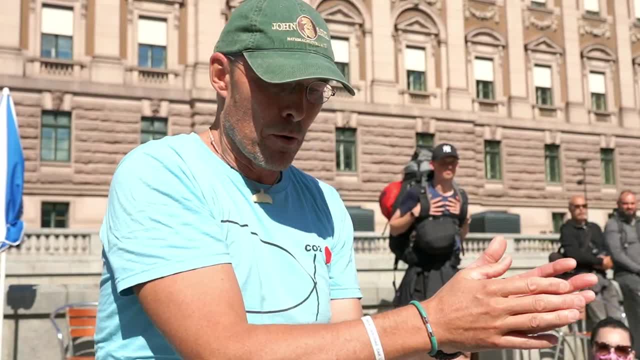 like Storglaciären Storglaciären, it's the most examined glacier in the whole world and the longest mass balance record since 1946. So a lot of researchers. they come to Tarfala in Kebnekaise. 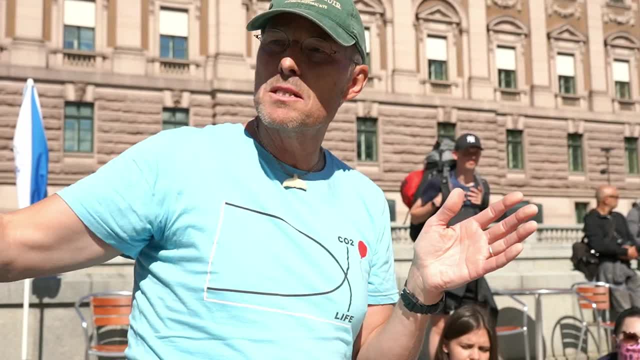 to study this glacier And they say: you know, this glacier is the most examined glacier in the whole world and the longest mass balance record since 1946. So a lot of researchers. they come to Tarfala in Kebnekaise. 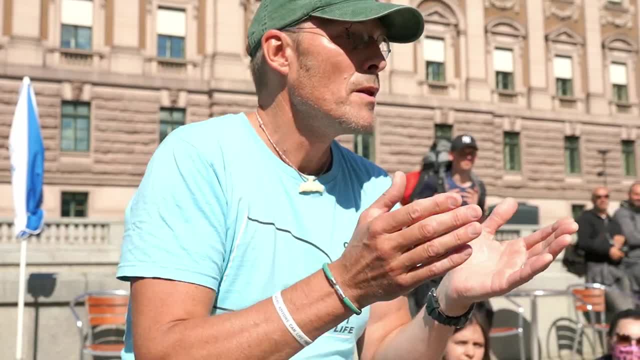 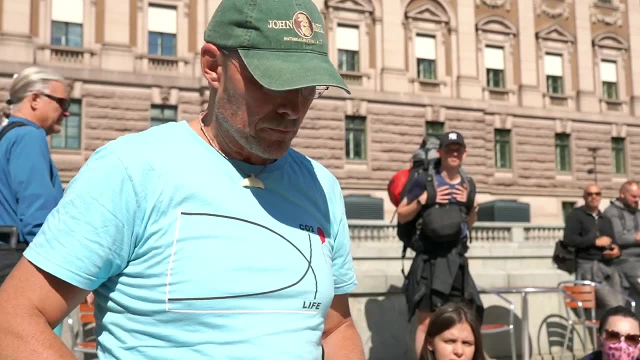 to study Storglaciären, because they know so much, we know so much about it, And then they can continue to do their enhanced research on it. And then you have Icefield or Plateau Ice, Piedmont, Glacier. it's like an elephant's foot. 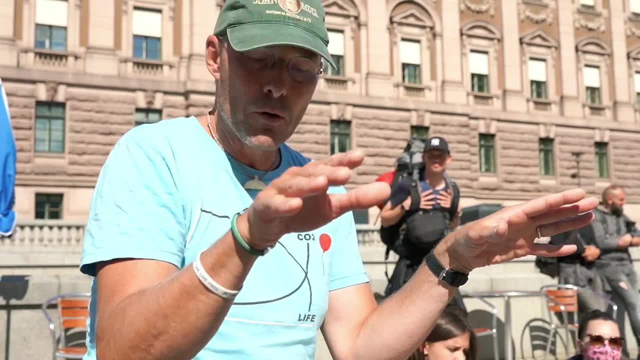 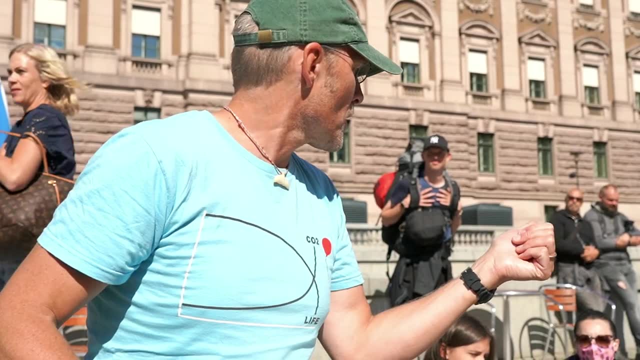 It's pretty cool. It's in Northern Canada, we have these Piedmont Glaciers, And then you have these ice sheets for inland seas in Swedish, And they are huge. Still we have Grönland and Antarktis. They come. 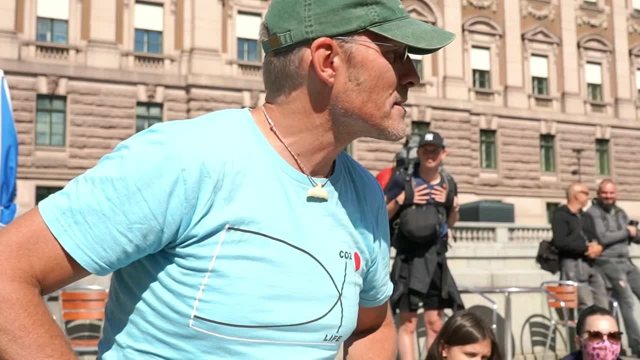 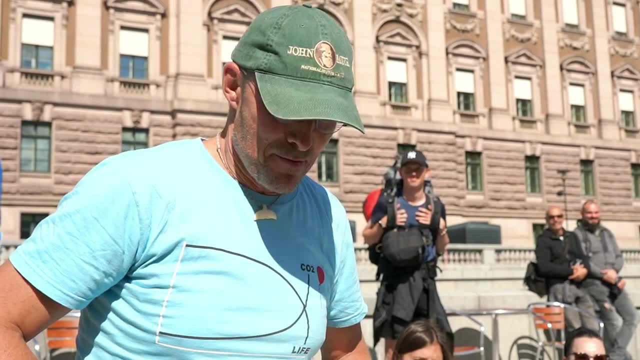 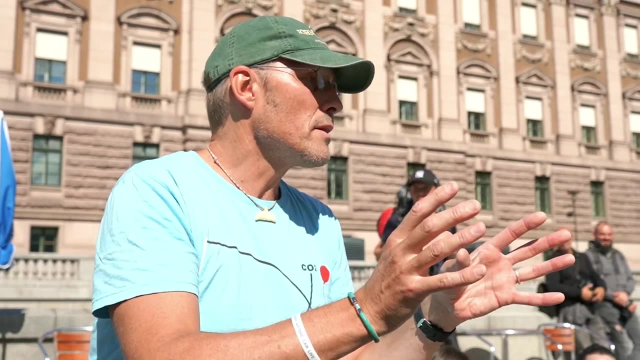 So why should we care about the glaciers? Well, I love glaciers, but I'm an ice nerd. So, but why should we care about them? Well, it's all connected: because our emissions, they create warm heat and the glaciers melt. 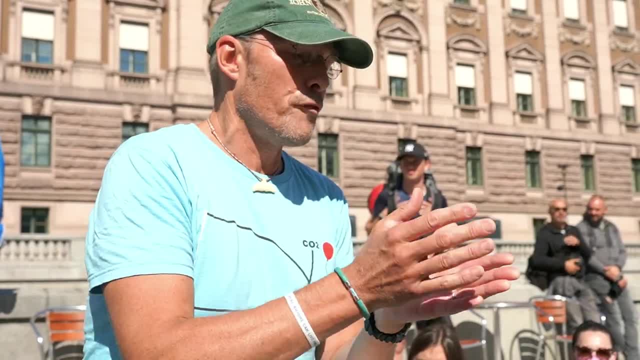 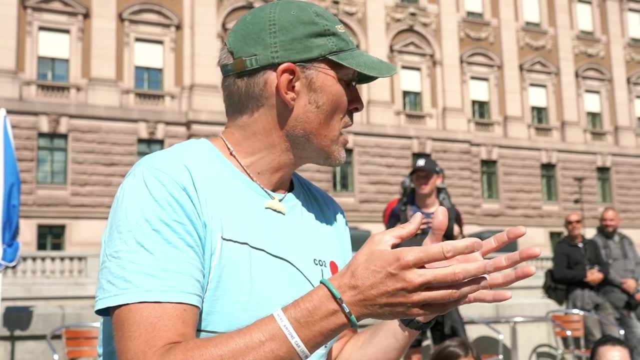 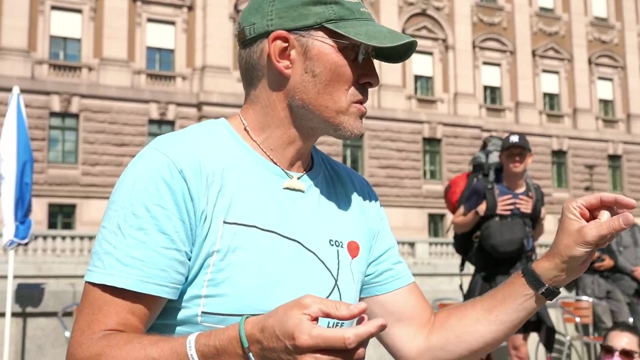 Just to compare, you know, the normal emissions of fossil carbon is about 1.3 to a half gigaton, a billion tons per year. We emit 40 gigatons, 100 times more than the natural sources. If somebody says 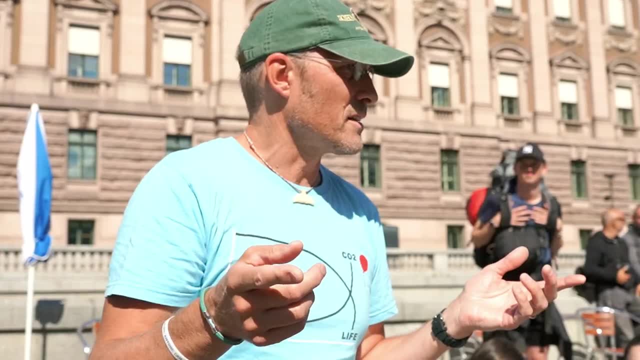 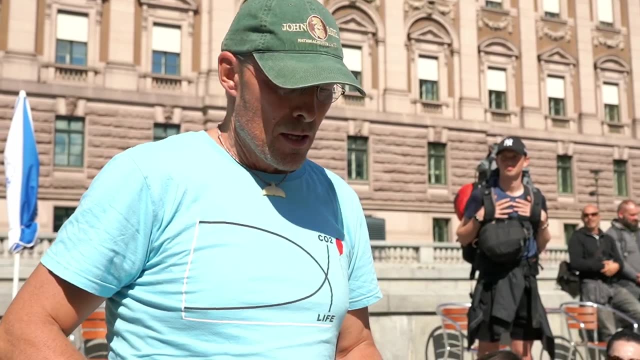 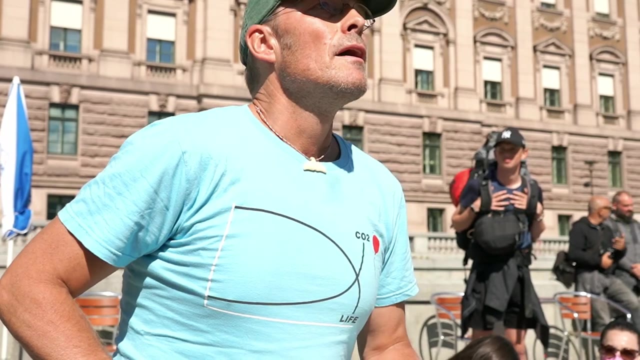 it's natural. the cold cycle, yeah, but we emit 100 times more than all the natural processes in the fossil carbon dioxide And that creates heat. I go to this. And if you see in Sweden these 250 glaciers, 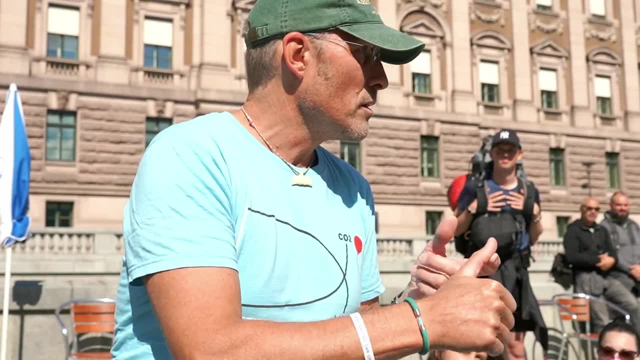 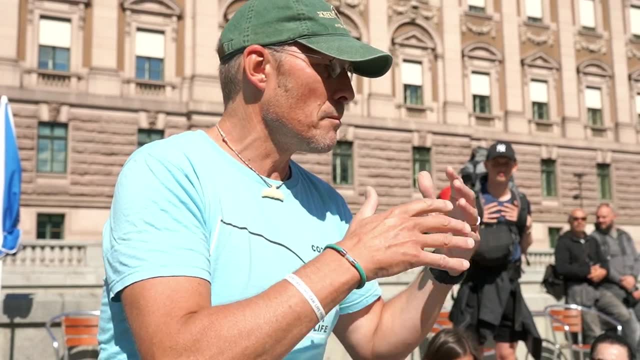 they create power, clean power for us, water for irrigation and drinking and also to keep the balance in the nature when it's dry. In other, in the Andes or even in the Himalayas. you know it's called the Third Pole Himalayas. 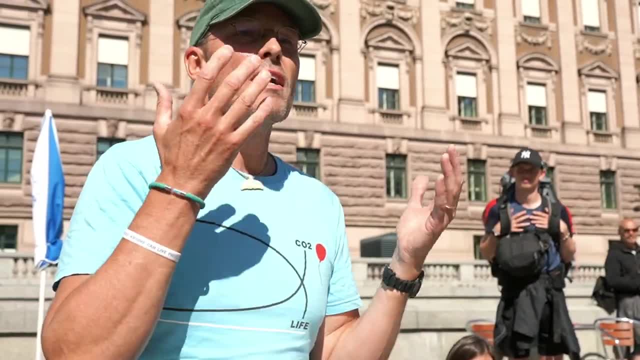 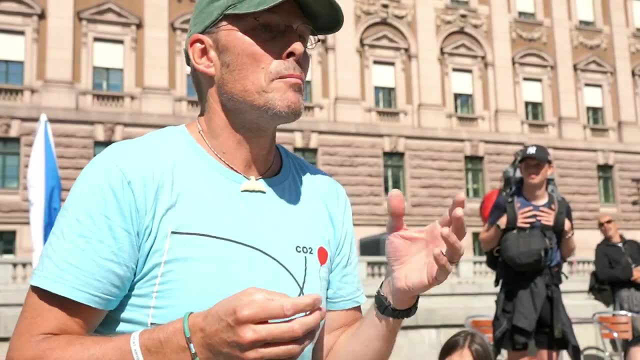 with Mount Everest, or Shumalungma as the Nepalese say. It's glaciers that you know. it's not just in the Andes, or even in the Himalayas. you know it's called the Third Pole Himalayas, with Mount Everest. 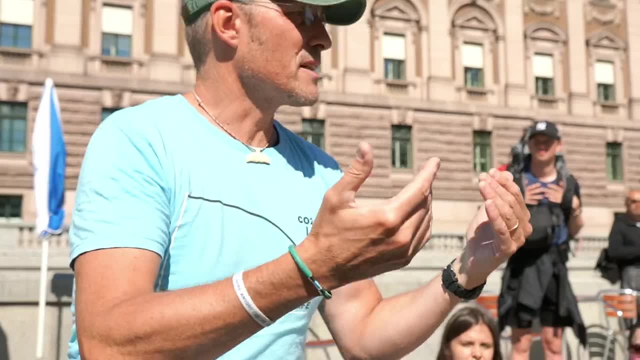 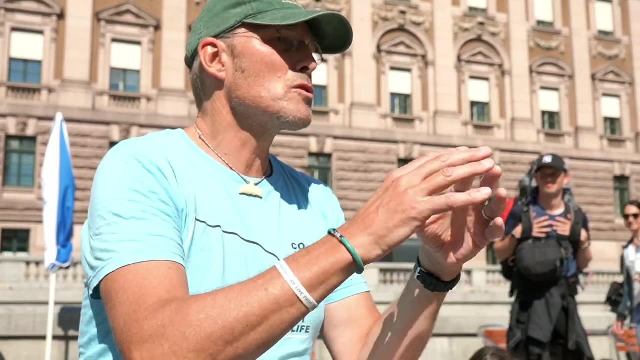 or Shumalungma as the Nepalese say. They are now melting so fast that you have this flood, flash floods, And they are destroying rivers, villages and also power dams And, when they are gone, if we continue, emit fossil fuels. 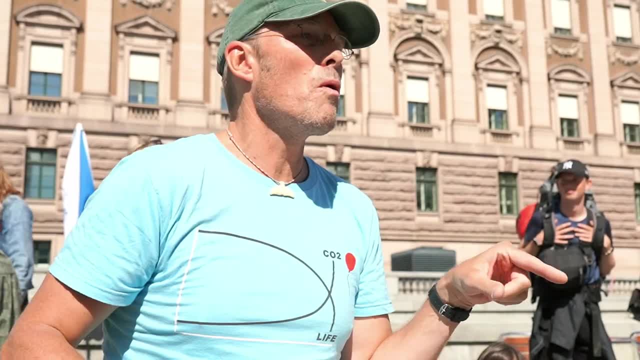 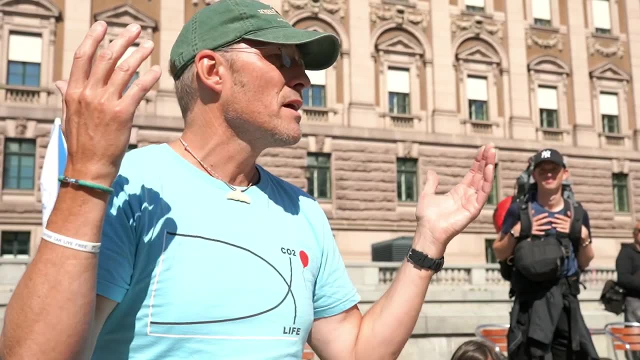 then it will be dropped, And it's about 1.7 billion people dependent on the glaciers And soon, in a couple of decades, it will be two or two and a half billion people dependent on these glaciers. So what should they do? 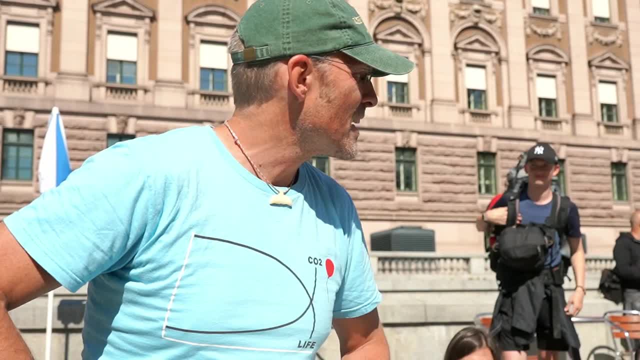 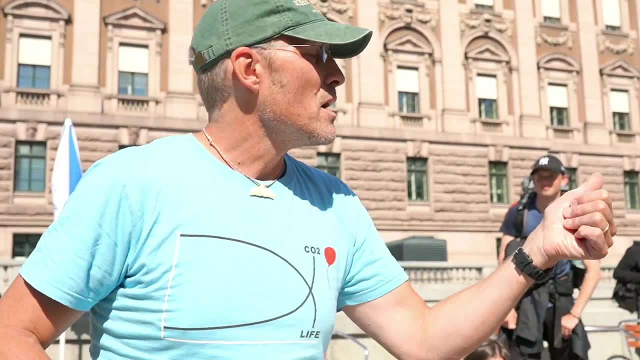 if they have no water for irrigation or drinking. Two billion people, Could you imagine, don't have access to water. You know, in the tropics they have monsoon and then they are dropped. They have no seasons like we have here, And when it's dropped 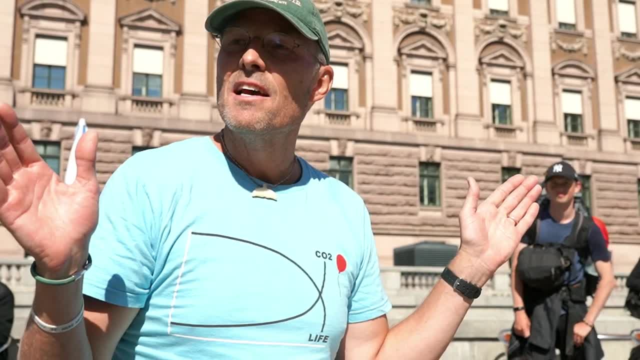 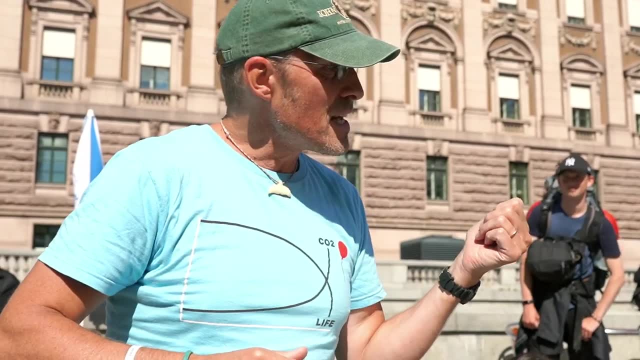 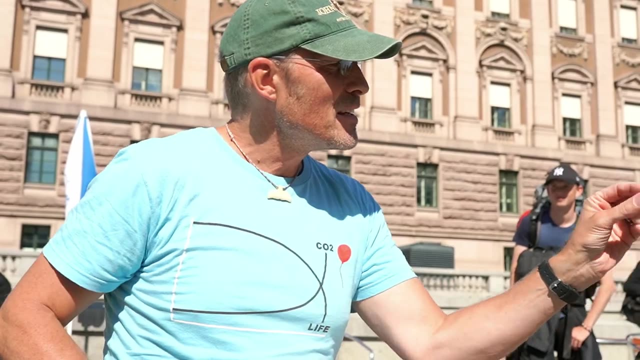 for half a year. they have no water. So everything is connected. you understand Our choices. every ton of fossil fuel we emit creates a worse situation for the glaciers and also for all those billions of people. So that's why a little super specific. 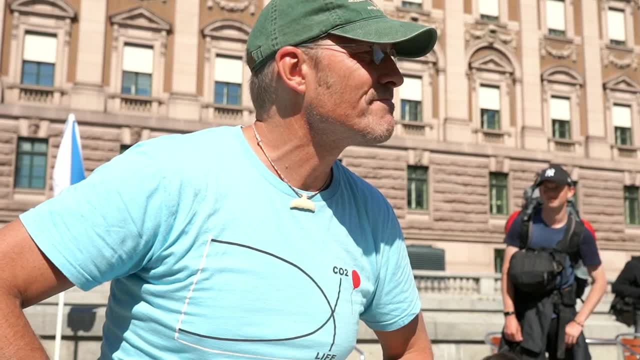 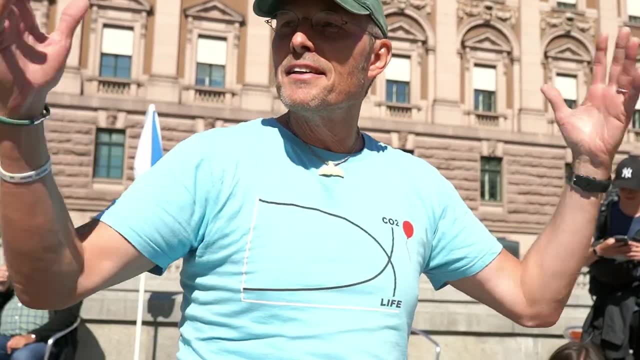 interest in ice is so important, I think I'll stop there. It's a lot of things to say. I could sit here for hours. I would like to. I would love to take you up to Storglansjärven to show you. 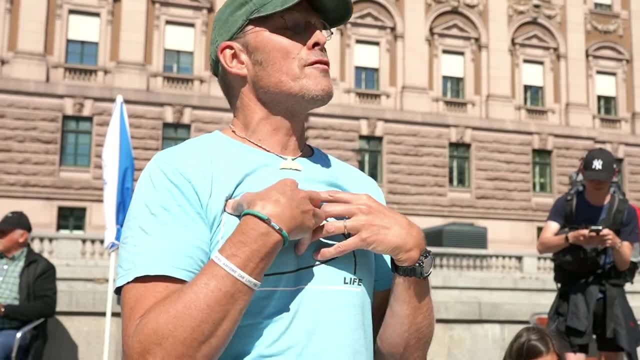 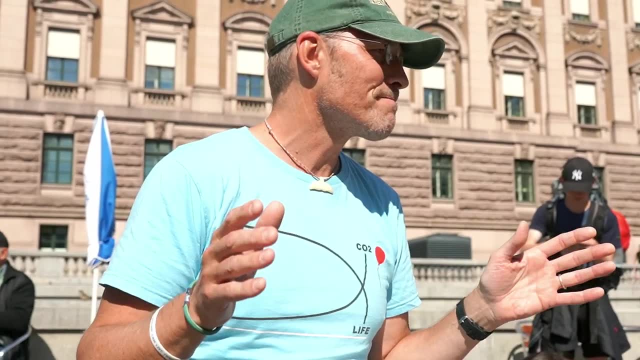 the beauty of the glaciers, the beauty of the crevasses in a safe way, because you really feel like you're alive. You get strong legs, and the food taste is marvelous And, if you're lucky, there's a sauna as well. So thanks a lot. 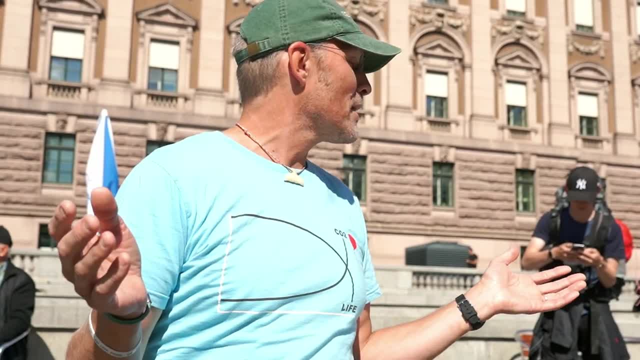 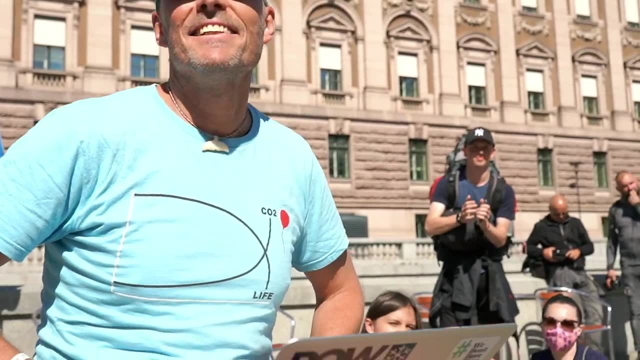 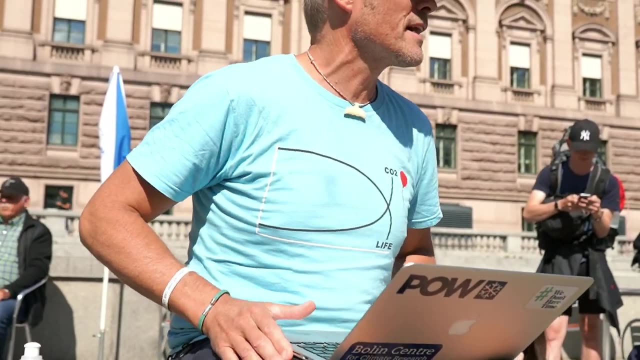 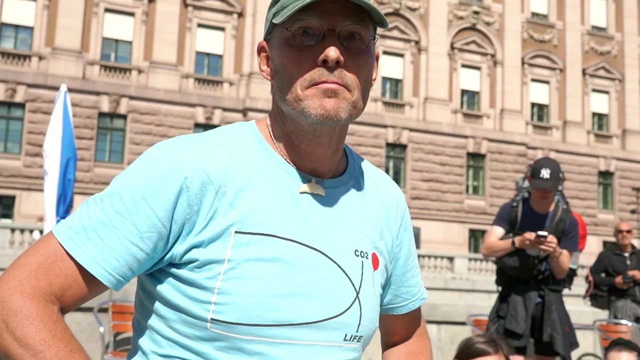 for listening and I'm eager to hear your questions about things that I missed. You can take it in English or Swedish and I can just repeat them. So because this is recorded for researcher's desk, so others can also listen to this, Yes, please. 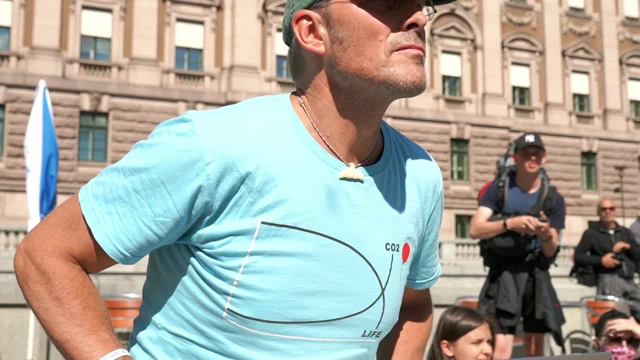 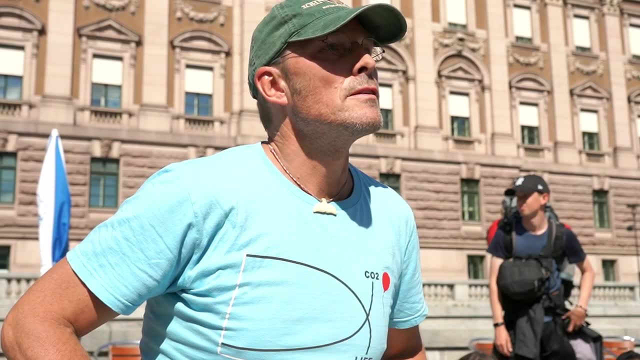 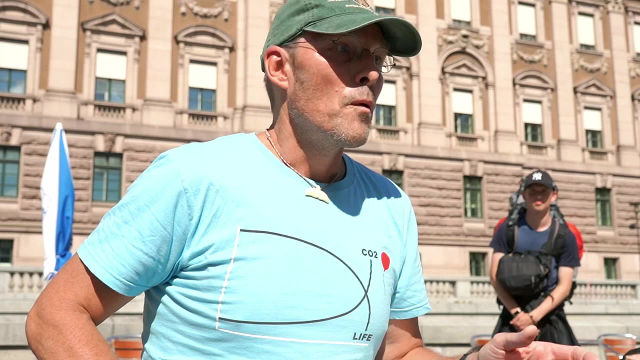 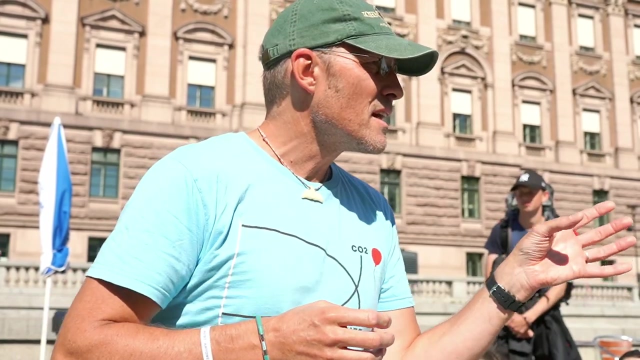 Yeah, yeah, that's a good question. How can we define the temperature when you're drilling the ice? Well, you see, oxygen creates some different isotopes. So oxygen 16, 16 per hour, per hour per minute. So when you're drilling, 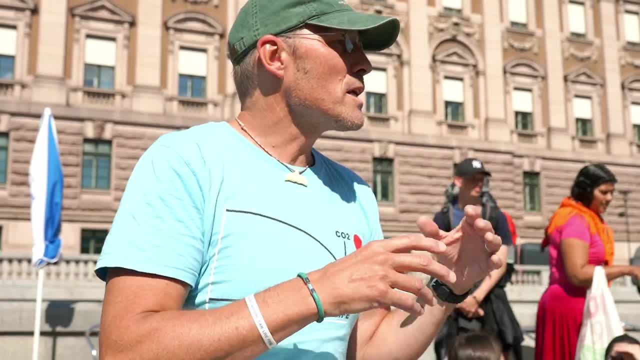 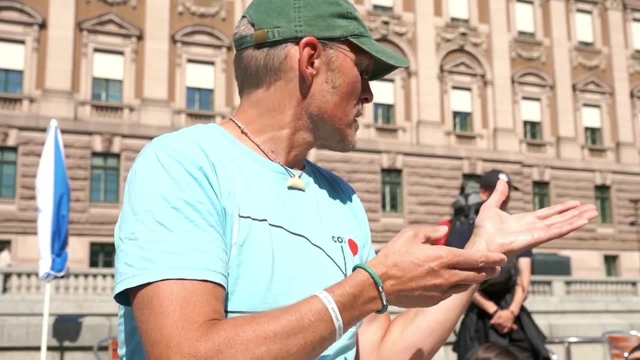 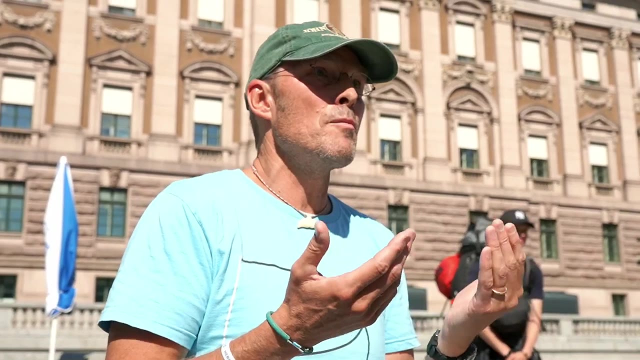 16 proteins, core particles. it's lighter than oxygen 18.. So when it's warm, you know, all the oxygen leaves the ocean. But when it's colder, only the light oxygen leaves the oxygen: 16.. So when it's more oxygen, 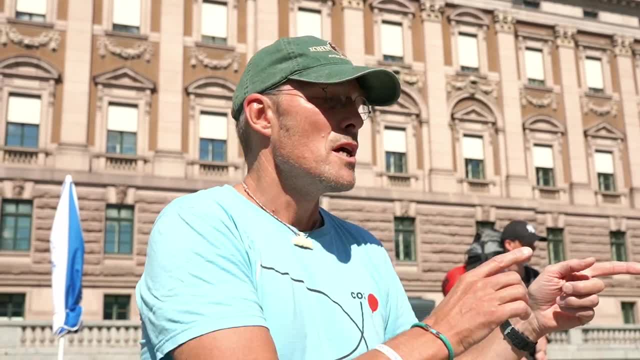 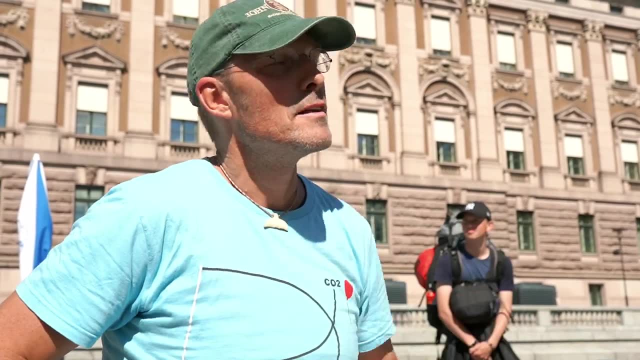 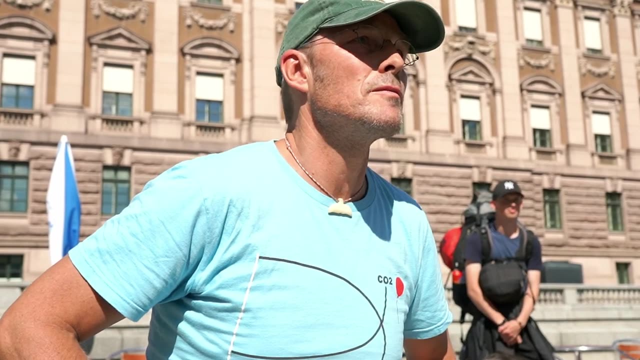 16, then it means it was colder. It's like climate proxies: You can check that changes back in time. But that's it. That's a good question. So the glacier is a perfect climate record if it doesn't melt. Yes, 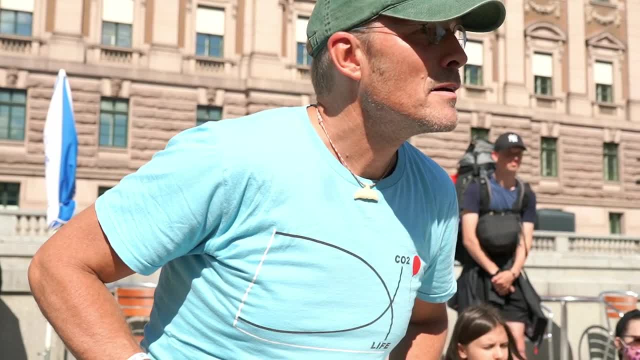 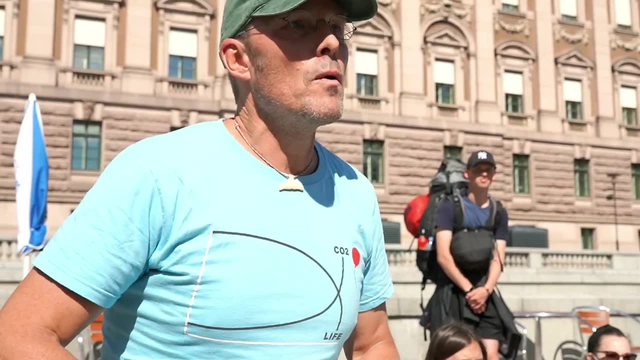 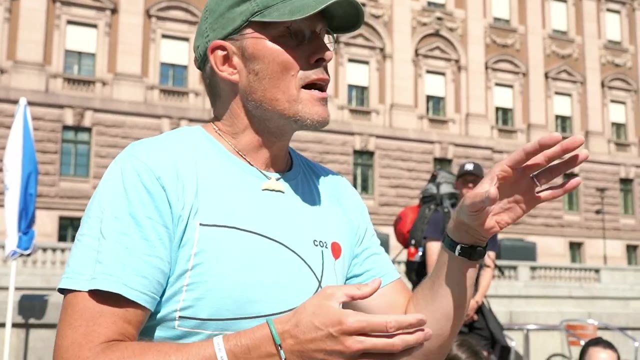 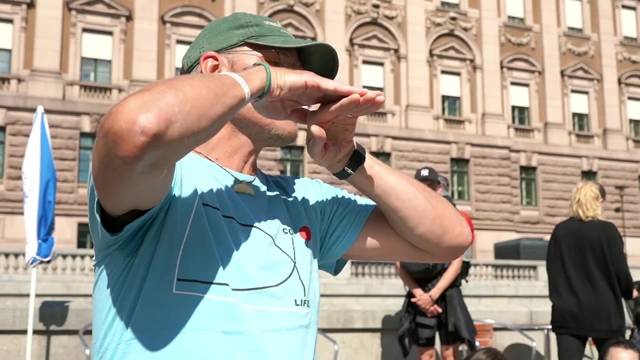 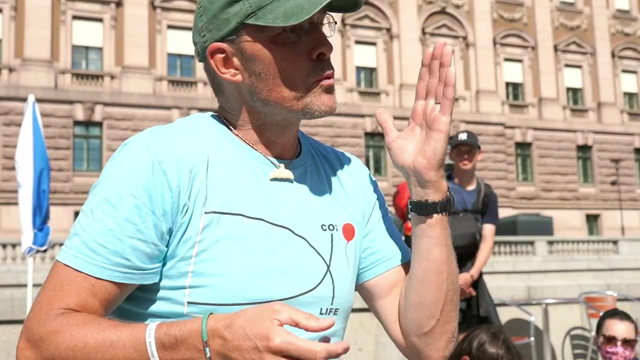 please Do you think that climate records are why she doesn't look here and look? because you use all kinds of the ice. You can miss some years because it can be melt, It can be sharing, like when the ice moves. Actually, sometimes you can. 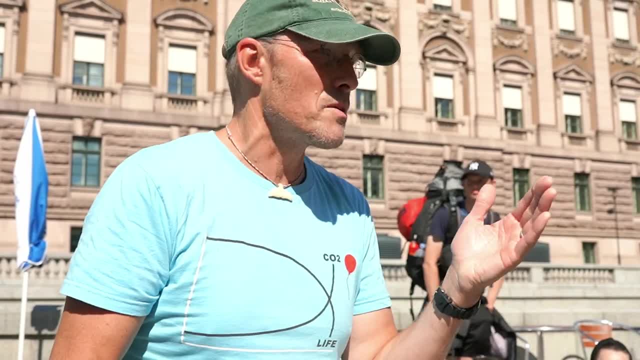 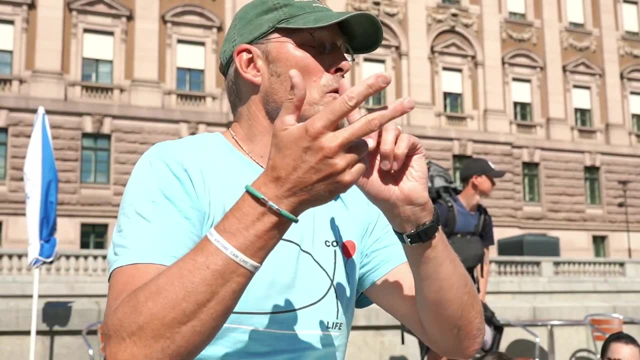 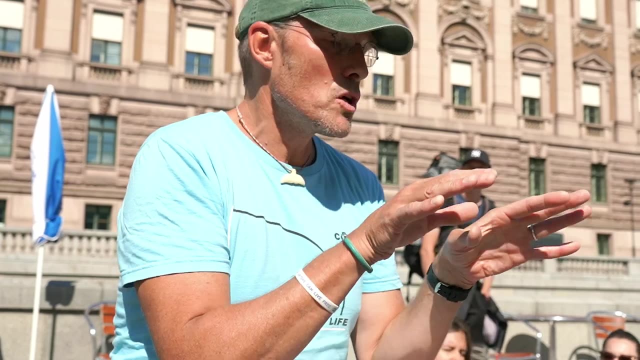 share like that, You have the opposite. So that's why we did this dynamic study. But with trees you can compare each year because it depends on temperature and moisture. So you can have these trees to compare with just to adjust the climate models. 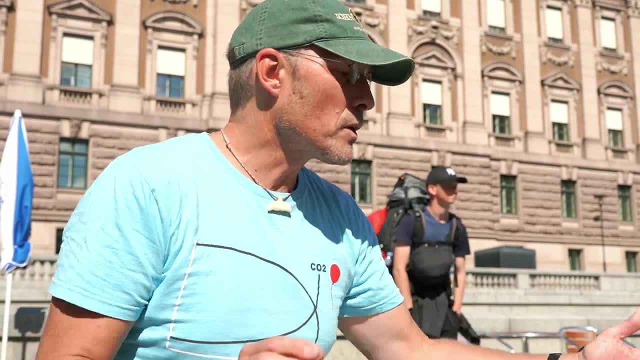 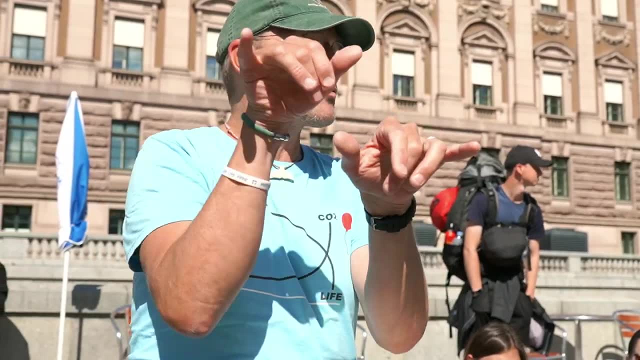 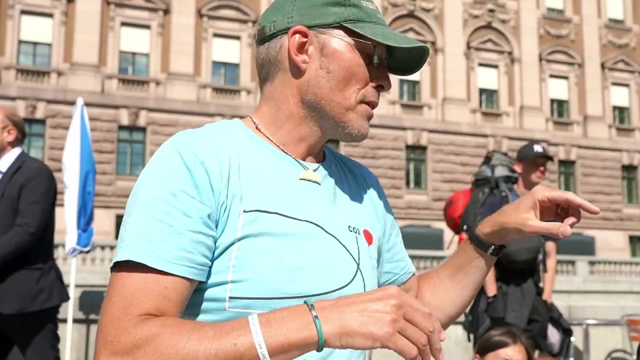 And you have these fossil trees in the pit box, for instance, They can be 10,000 years old and you can drill in them and you can measure. through the trees, you compare to the glaciers, and then sediment cores in the lakes, And then you 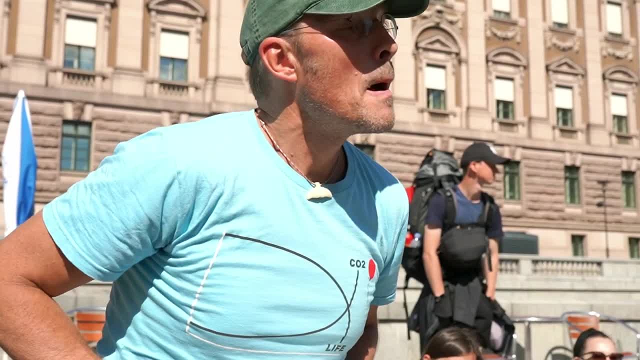 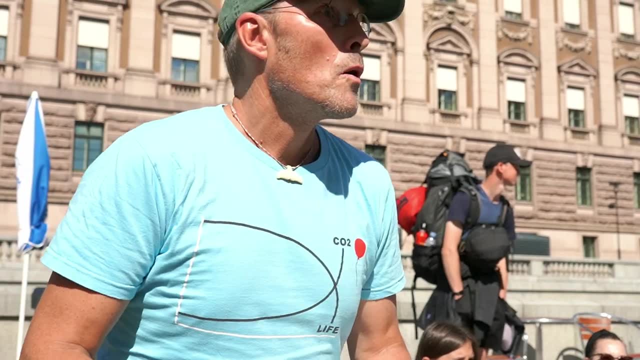 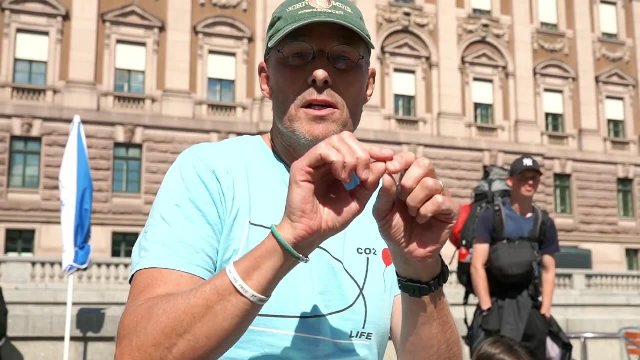 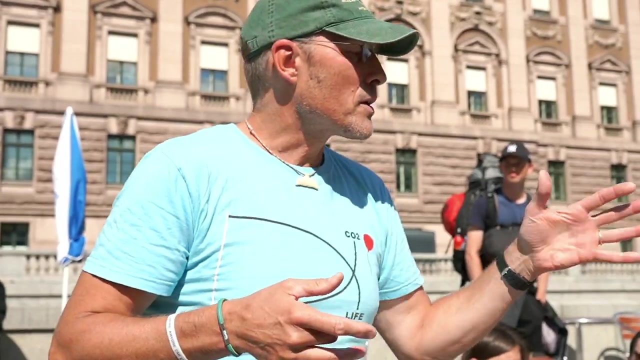 create these patterns You need a lot of data. You cannot just take one record and say: this is the fact. Yeah, you can do that. Yeah, if you compare, how do you compare this? if you look at the volcano eruption in, 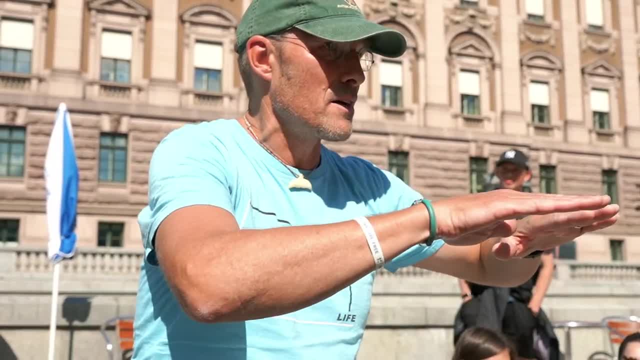 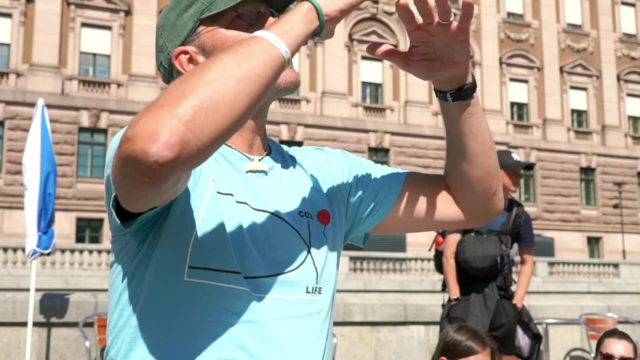 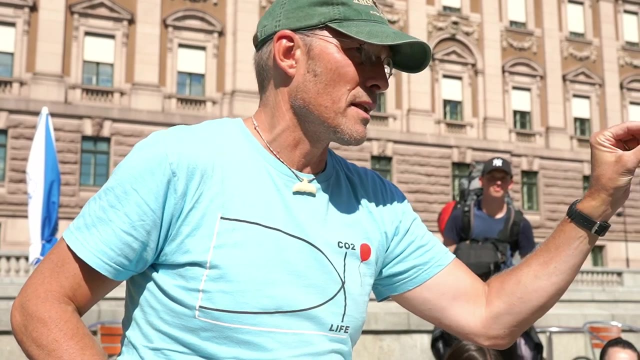 Krakatoa in- I think it was 1883, you can see a lot of ash layers all around. all glaciers have these ash layers, Also sediment cores in lakes, And so you can also see that it was colder by then because the ash layer 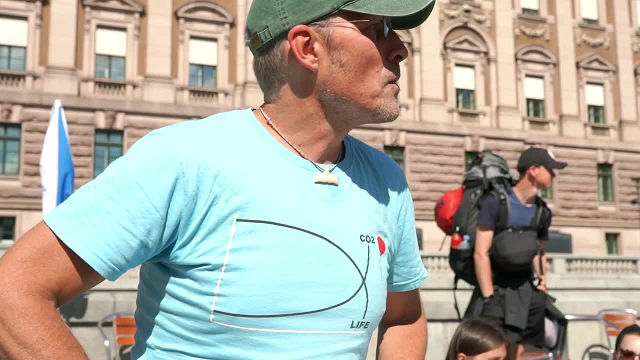 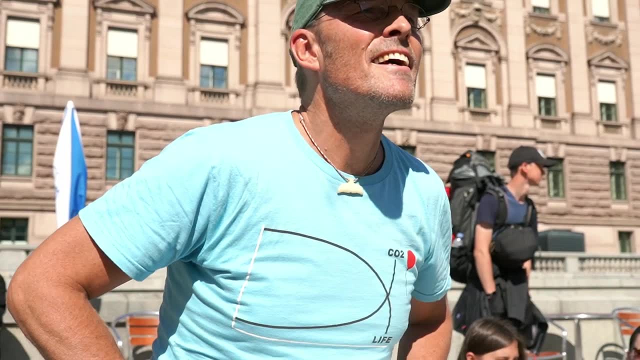 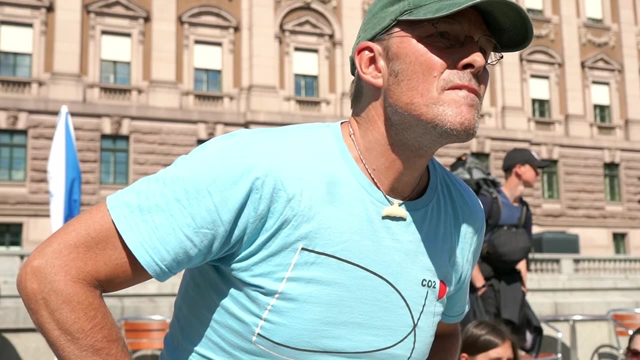 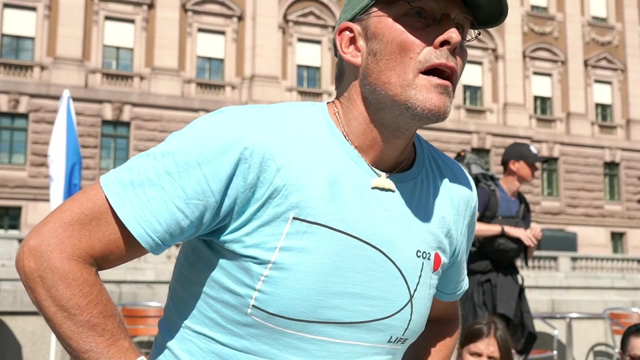 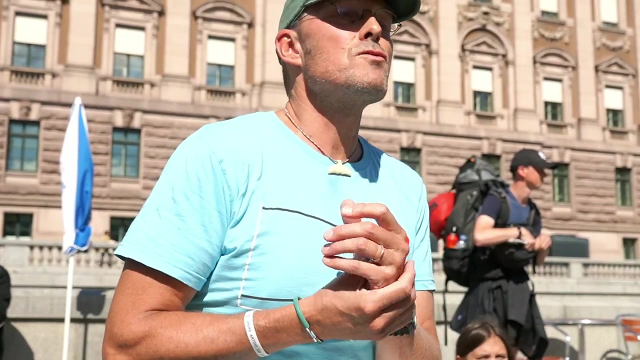 has these records. So it's a. you have to co-work with a lot of different scientists. Yes, please, Yeah. What's happening in Antarctica right now? It was a question about Antarctica and it's really cold, Like in the winter. 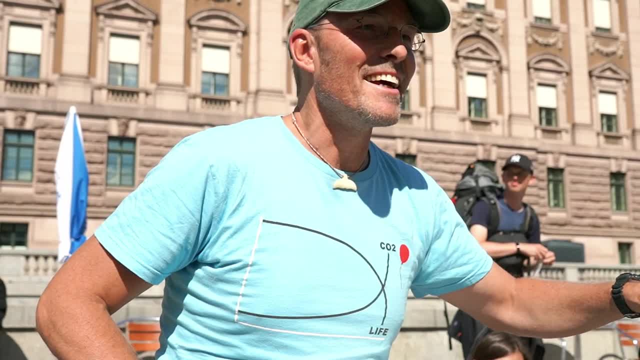 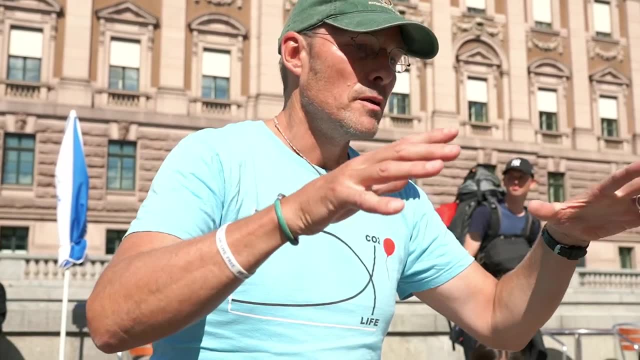 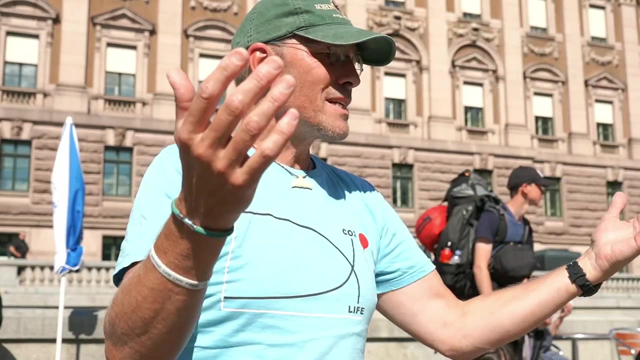 it's maybe 85, 90 degrees Celsius below. Don't go outside, You will. your spit will freeze before it leaves the mouth. So it's pretty cold there. But so actually some parts of Antarctica is growing because the surrounding seas 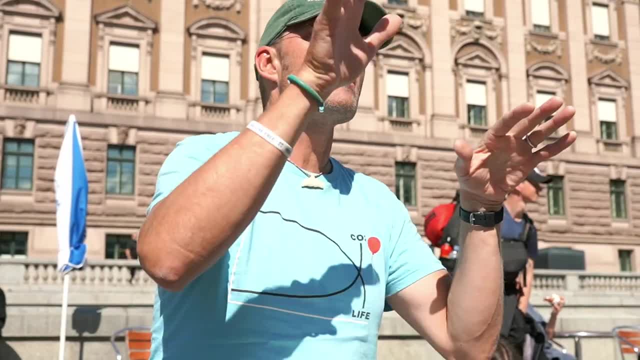 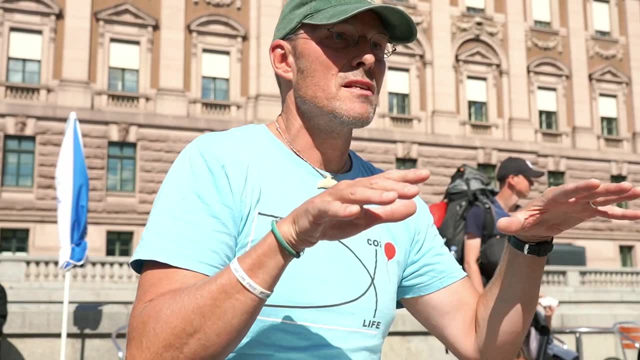 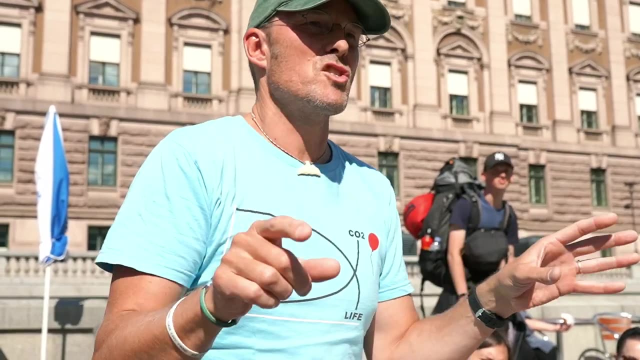 the atmosphere And when that moisture comes into the Antarctica it freezes as snow. So actually some parts of Antarctica is growing or growing. You can see that through satellites. but the melting in the fringes, like in the ice shells, it's so much. 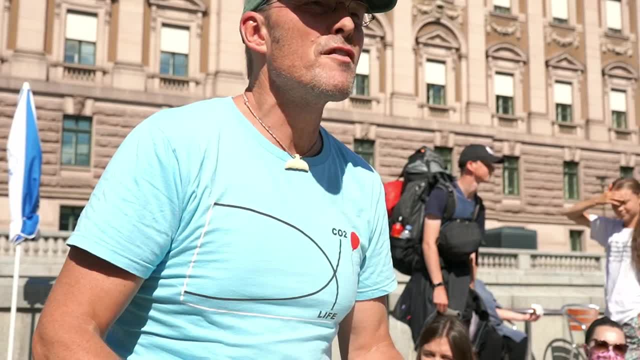 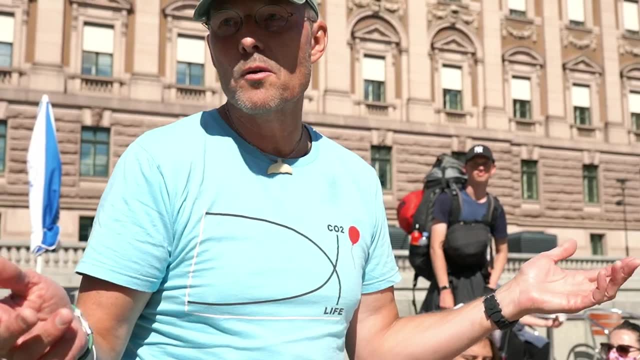 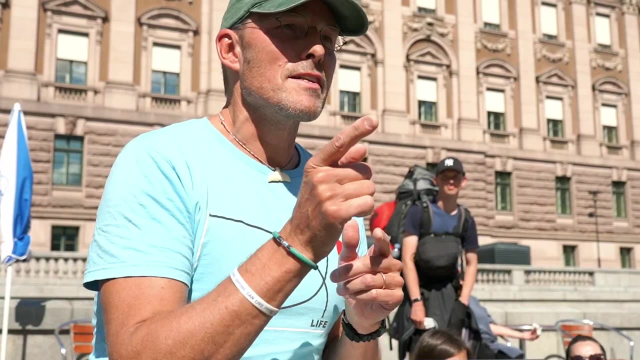 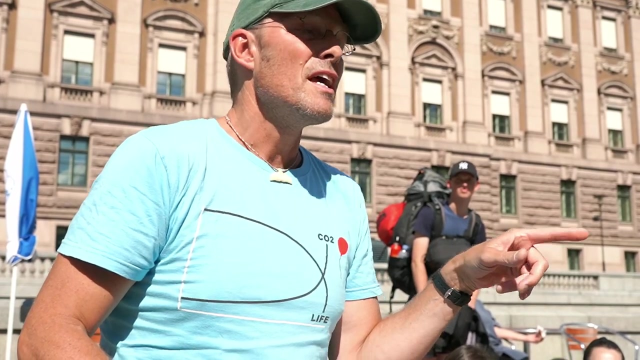 more, so that you have a pretty awesome negative mass. so if somebody- you know, there's some climate deniers or whatever we should call those factory system- they say that Antarctica is growing, and they are right in one sense: Some parts are growing. but the melt is so much bigger. The melt- net melt- is 150 gigatons per year And the next step for the future is that Greenland is probably lost. It will take hundreds or thousands of years, but it's probably lost Antarctica. 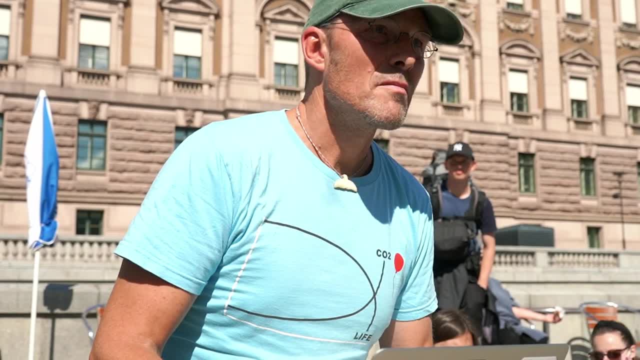 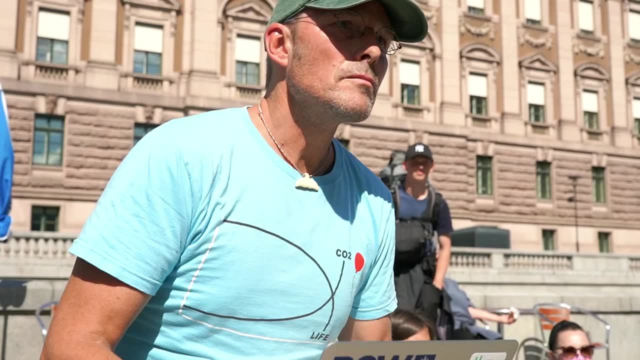 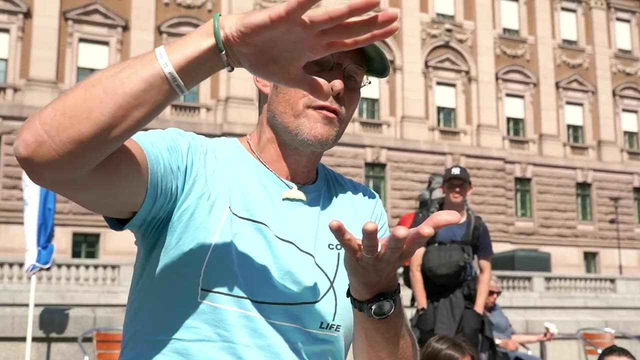 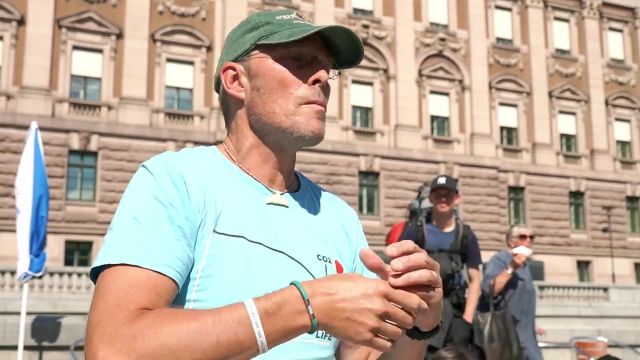 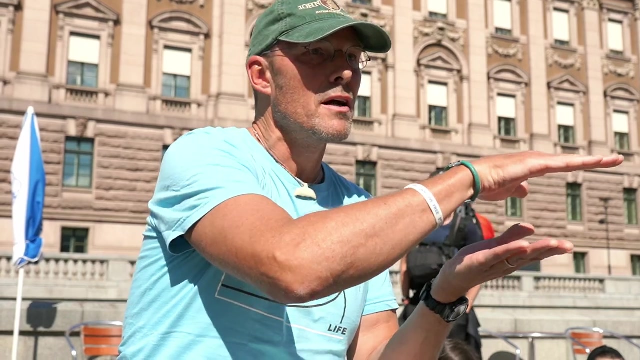 might be safe, but it depends on us. Yeah, Yeah, it was quite interesting to see the question about the ice shelves And ice shelves. it's kind of inland ice or ice sheets floating out, and it can be several thousand meters thick then it. 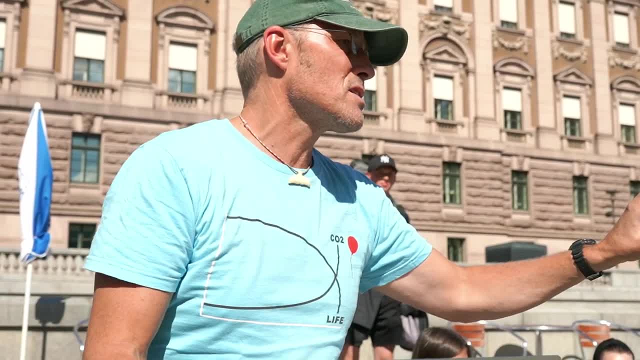 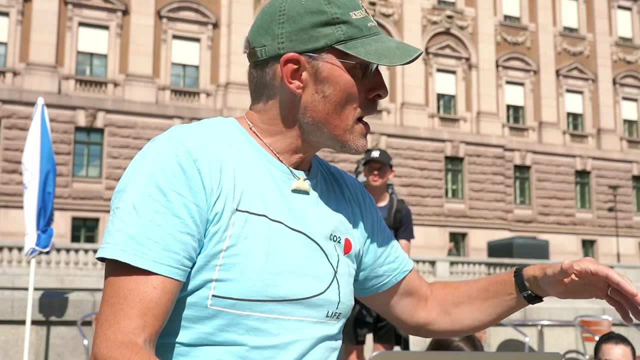 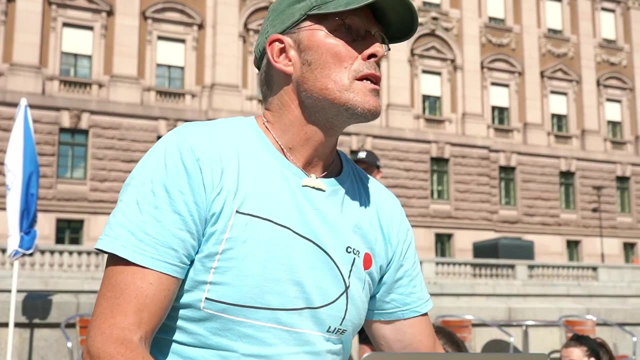 as soon as it reaches water, which has a lot of thermic power, as you can see, because ice is 10% lighter than water. so 10% is above, then 90% is below and there's a lot of melt below and that melting below. 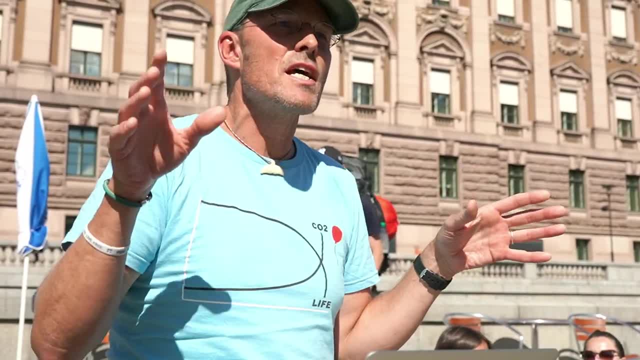 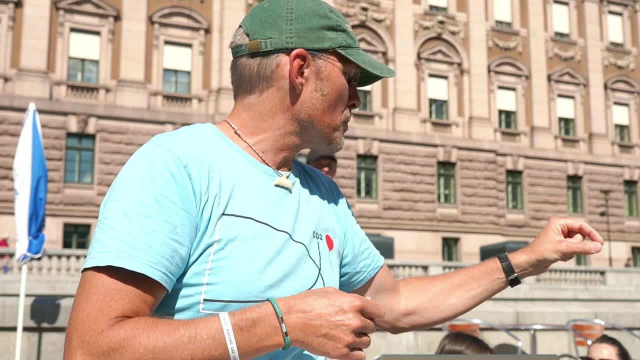 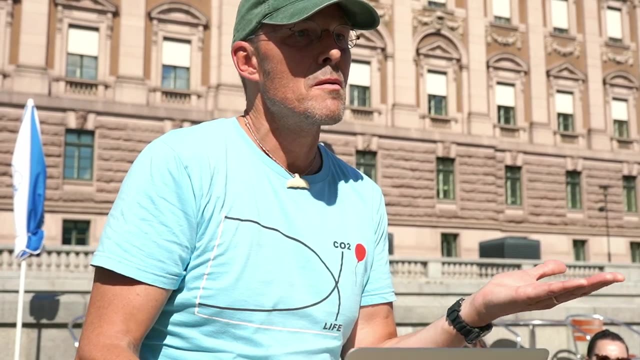 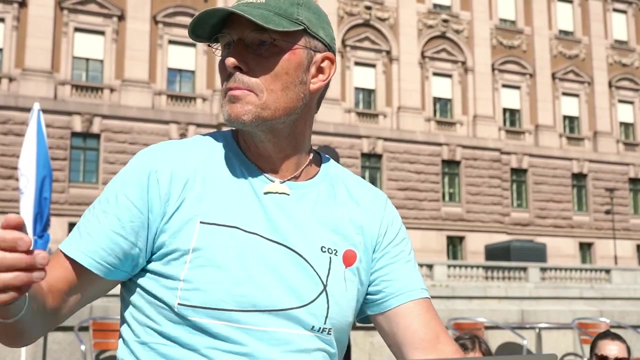 we have. researchers have missed that in many years so they have predicted that: oh, Antarctica seems pretty stable. it's probably growing a bit from below. you don't see that from the surface, but now they know, so they have to adjust all the models. Antarctica is melting so much. 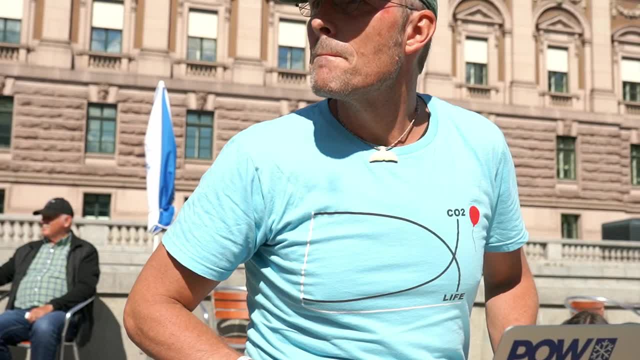 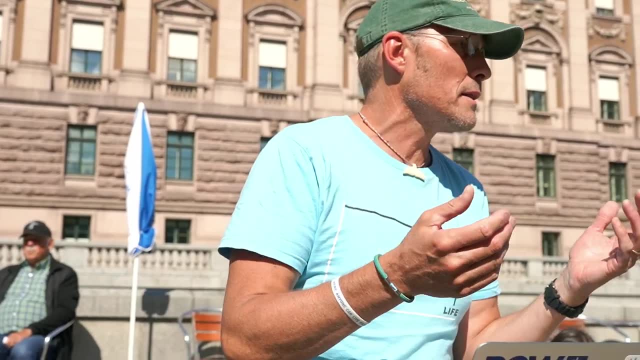 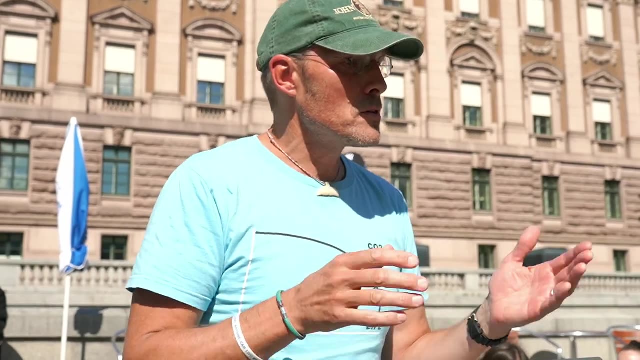 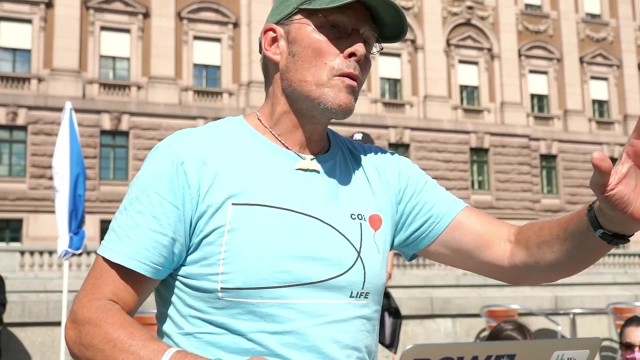 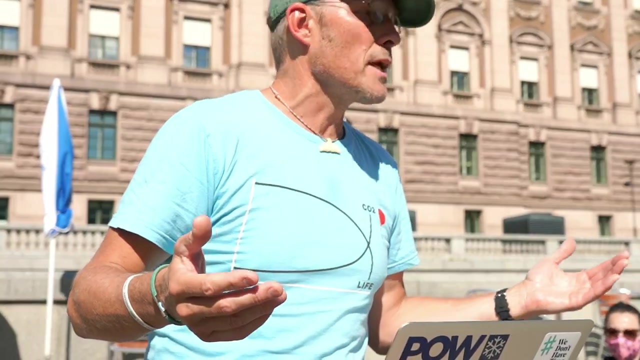 faster. yes, please, yeah. yeah, she asked the gulf stream and the melting of the glaciers. that's a good question. thank you, good one. you see that the gulf stream is starting in the Caribbean and it's bringing pretty warm seas water up to here. that's. 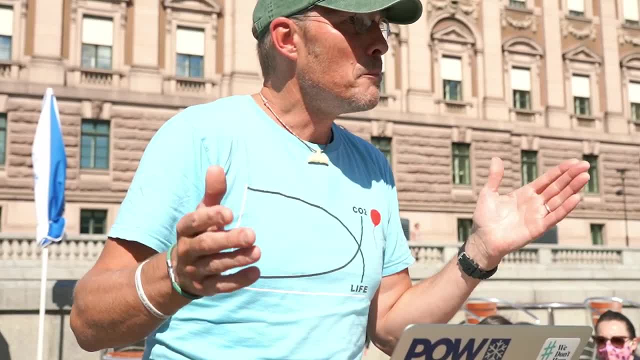 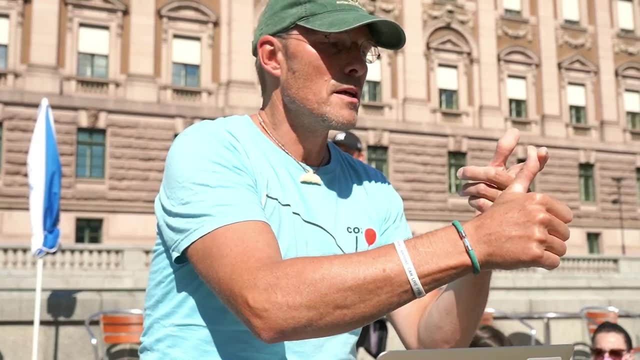 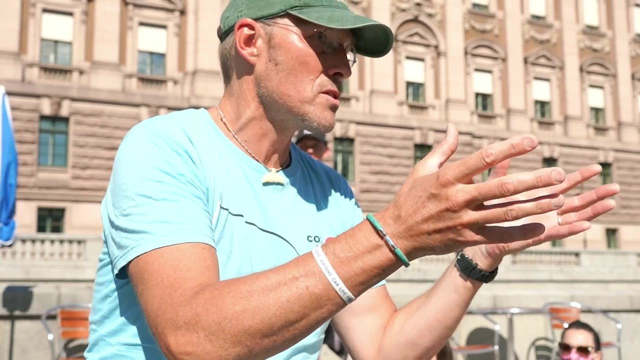 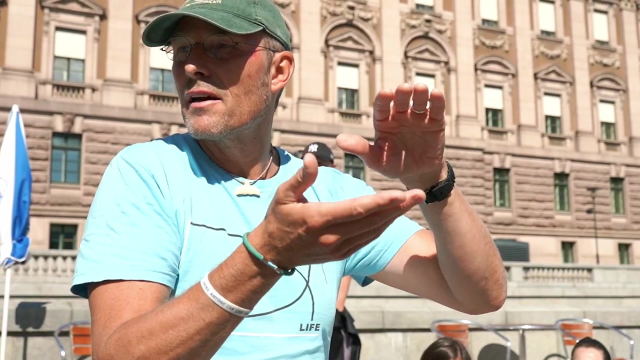 why we can sit here if we didn't have the gulf stream. the Arctic sea ice- and especially Greenland- is melting so much- 280 billion tons each year- so that you have this fresh water. and you know salt water is heavier than the fresh water. so when? 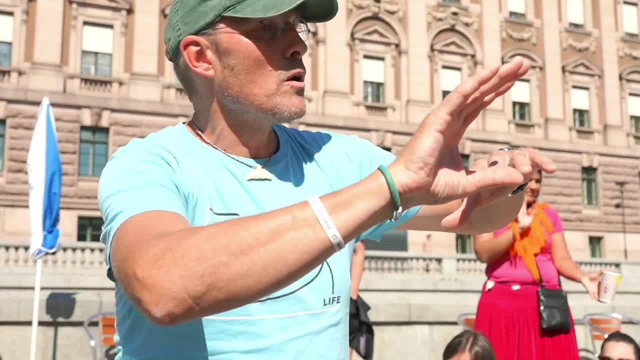 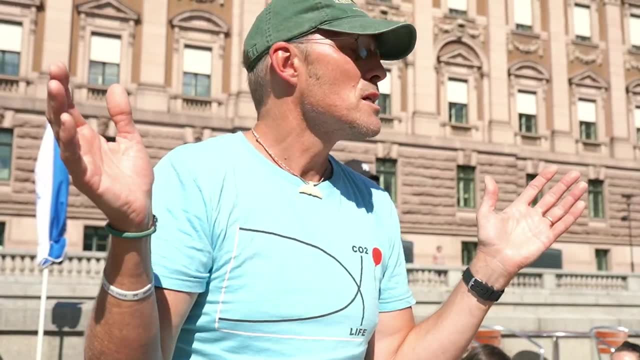 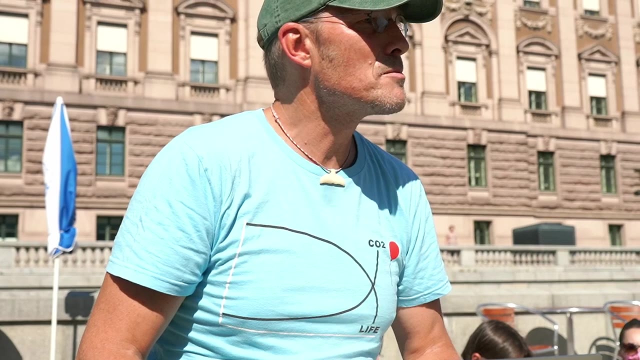 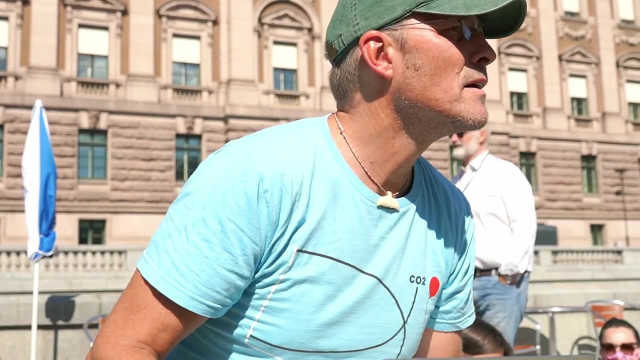 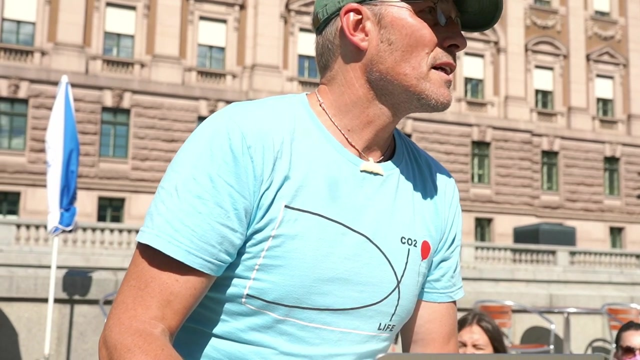 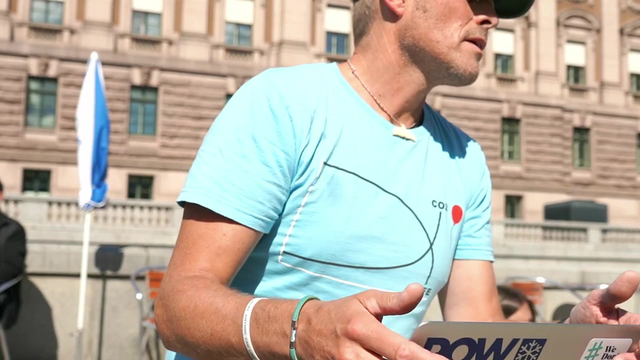 this salt warm water comes from the south, much further south, and that can create a cold spell here. so we, because of global warming, we could have much more colder in Scandinavia. it's pretty strange, but that's how climate dynamics works. yes, please, yeah, yeah, yeah, good. 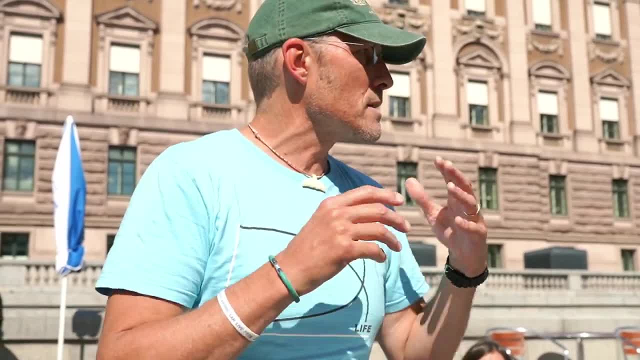 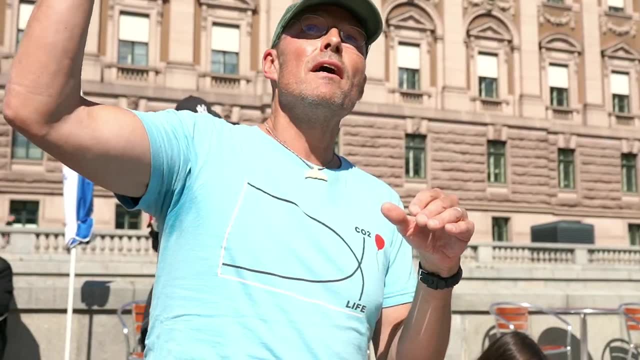 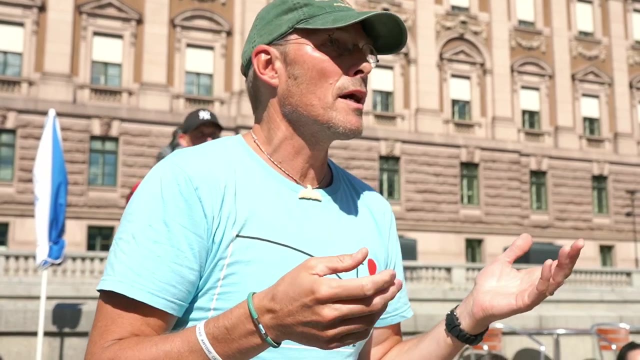 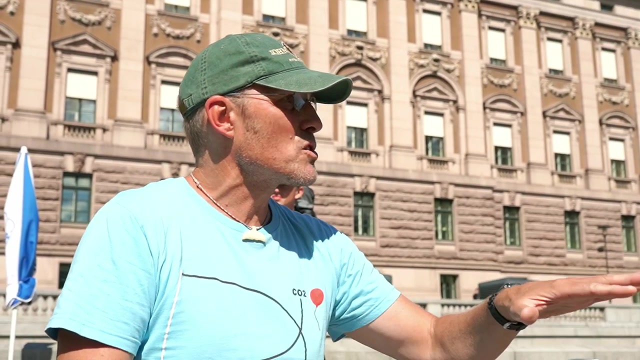 question. they talk about the albedo changing because if it gets colder then probably the glaciers can grow and we have more snow. and we have more snow, it reflects back the UV radiation. so if we can change the albedo to more light surface than dark, for instance, 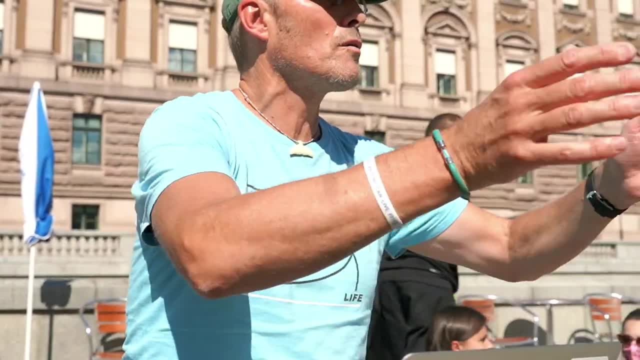 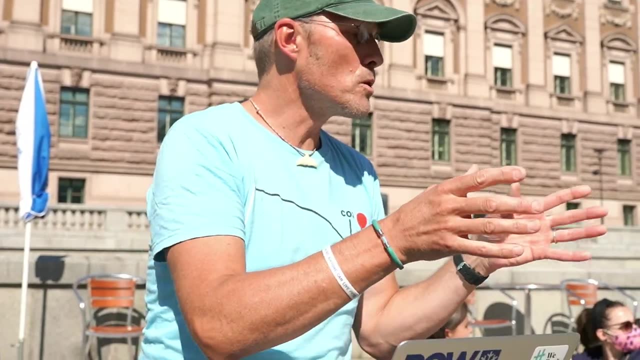 if you have a dark forest, then it creates a lot of heat. so, for instance, all this, when we plant a lot of you know, in the forest industry we plant a lot of coniferous trees like pine trees and spruce. then they are dark. it gets warmer. 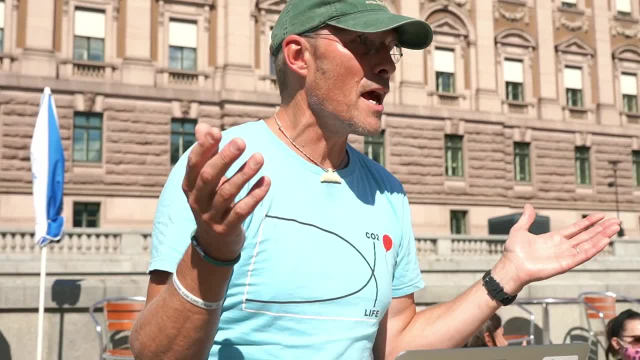 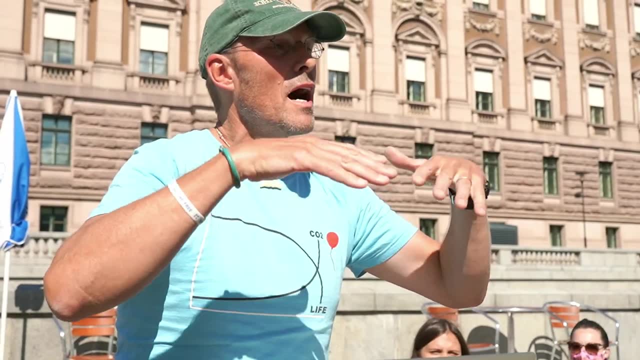 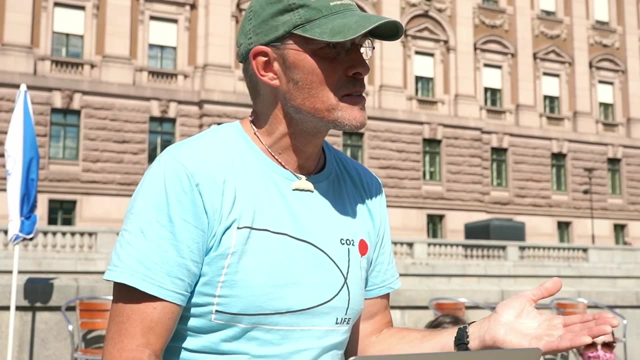 so that creates a warmer climate in Sweden if we would let the albedo and oak- it's more, much more lighter leaves, and that would create a higher albedo- reflect more back. so we should let nature take care of the forest, not the forest industry. that's also. 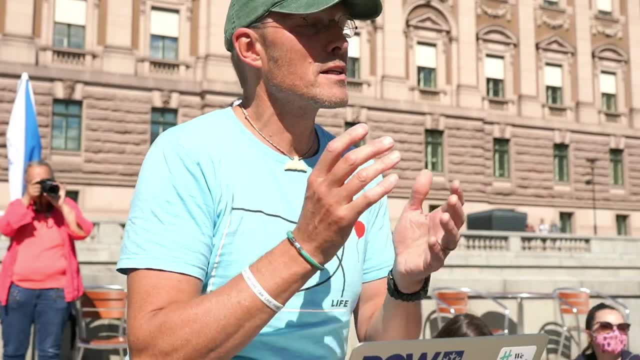 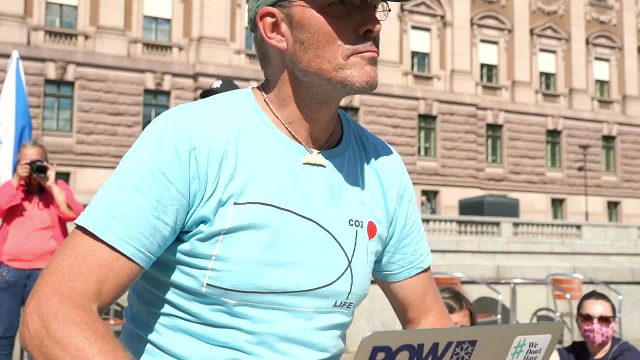 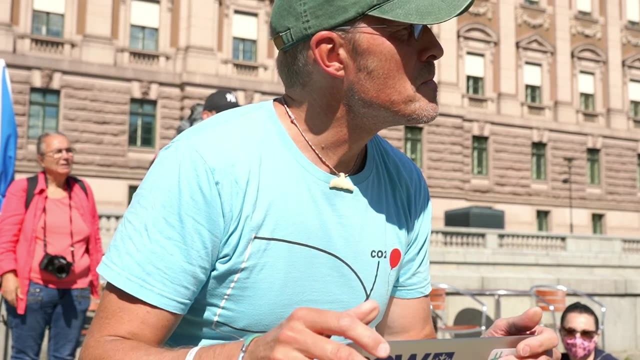 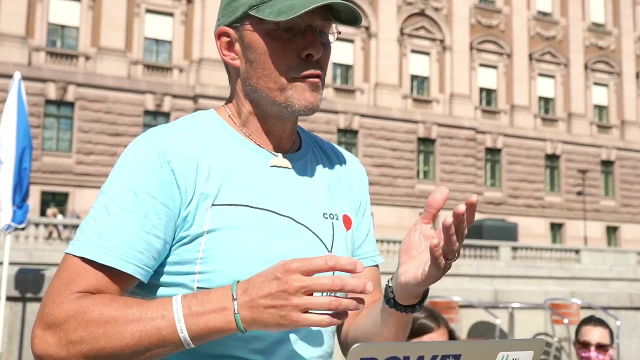 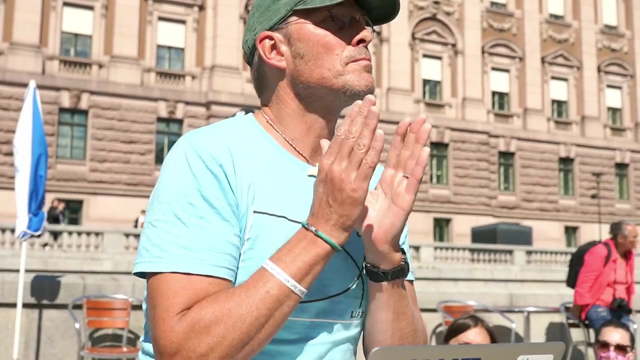 creating a climate impact. so you see, everything is connected. whatever choices we do affects the climate and our environment. yes, please, oh, that's a good question. she was asking that if the slowing of the gold stream was actually slowing down or affecting the carbon uptake. I have to pass. 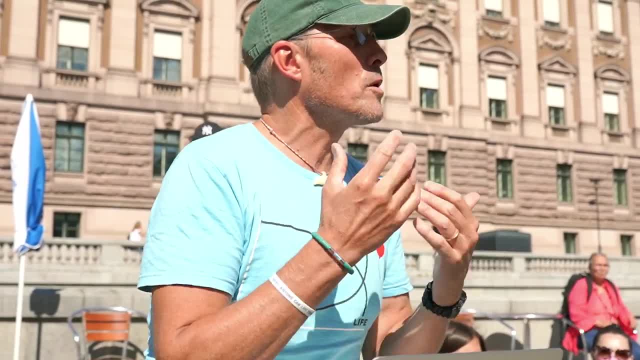 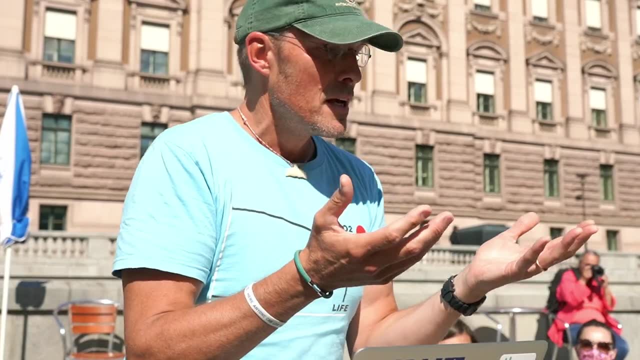 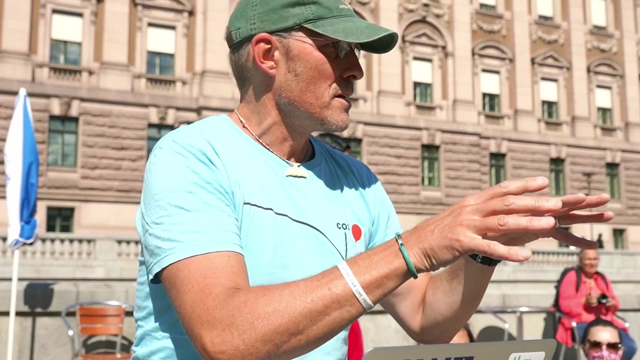 on that one, because it's a very complicated manner, because you have the uptake of carbon in the oceans. it has always helped us so that carbon dioxide resolved in the oceans, but it also creates, it buffers the carbon dioxide, but now it's saturated with carbon dioxide, so you have 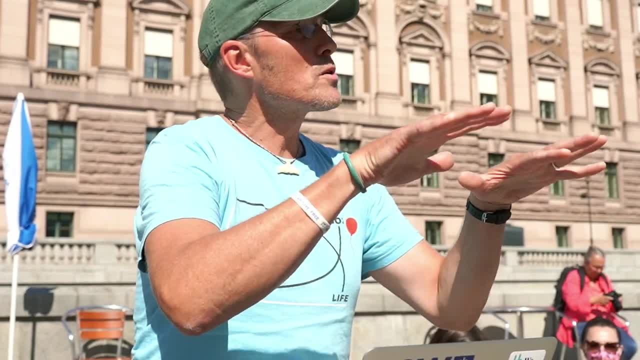 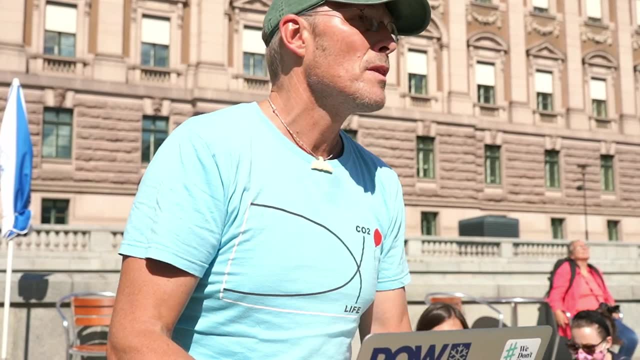 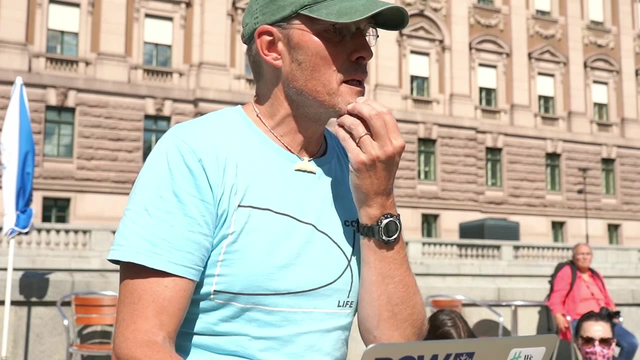 such a high level of carbon dioxide with an acidic gas, so the ocean is getting more acidic and cannot buffer any more carbon dioxide. so I would say that two to three times more in the arctic. so I would say that the possibility for the arctic ocean 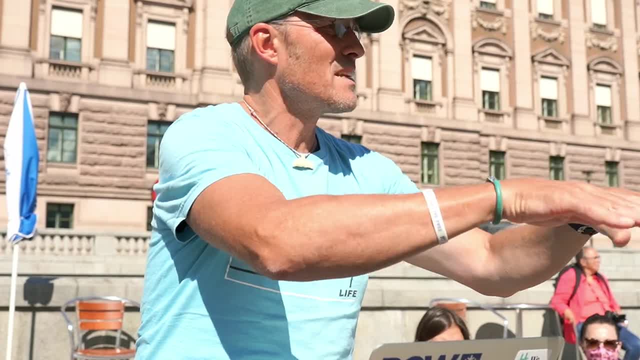 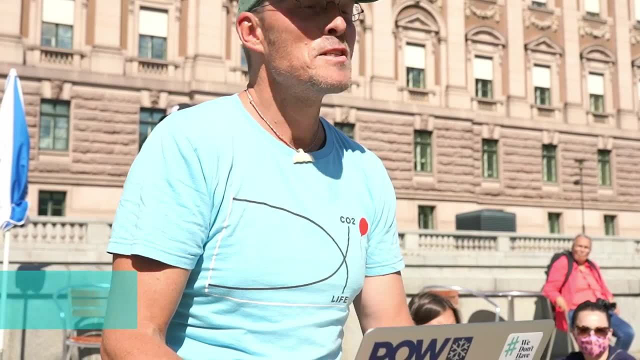 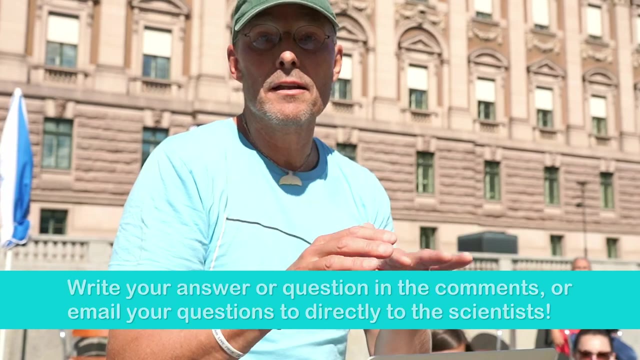 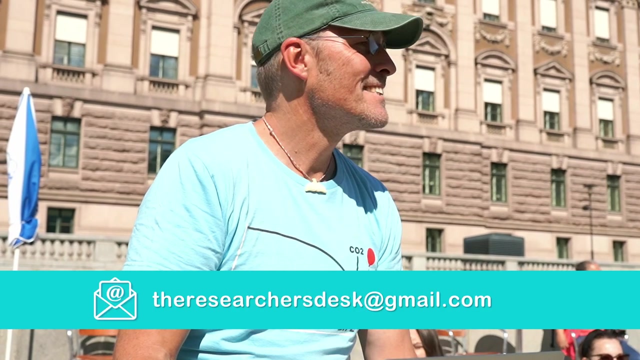 to sequester and take up carbon dioxide getting worse and worse, lesser and lesser. how that is affected by the gold stream is hard to say. maybe somebody knows, so please comment in the video on the internet. if you have any questions, please let me know in the comments. 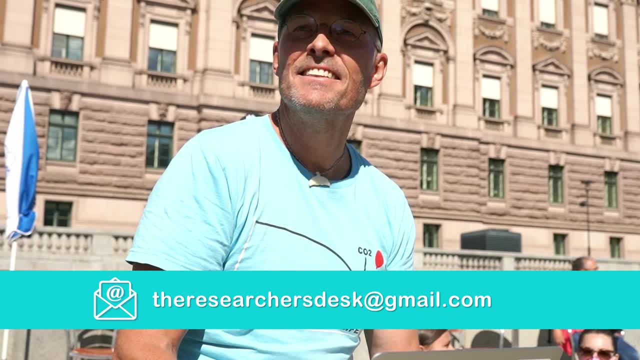 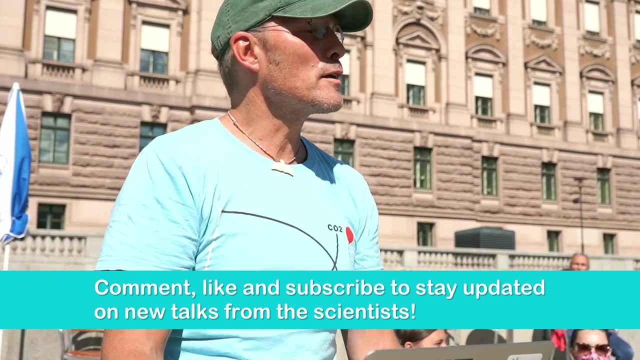 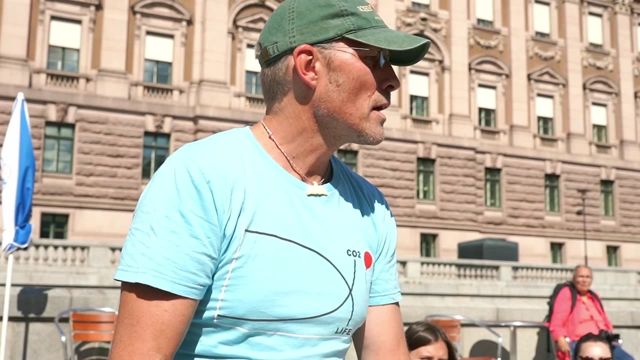 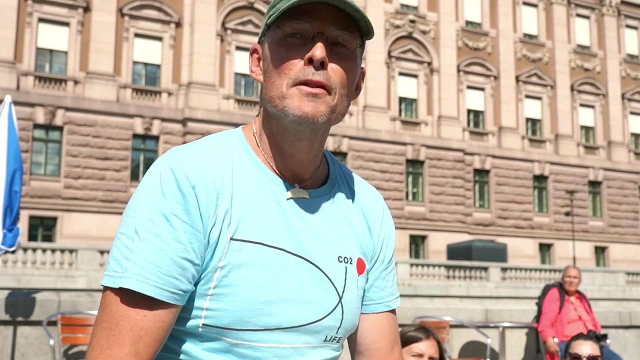 I will be here for a while I was. I will have a coffee with Toya and I will sit here. I can show you graphs and stuff. so if you want, you can come up just to talk and discuss whatever. Swedish, English, French, German, Skånska.